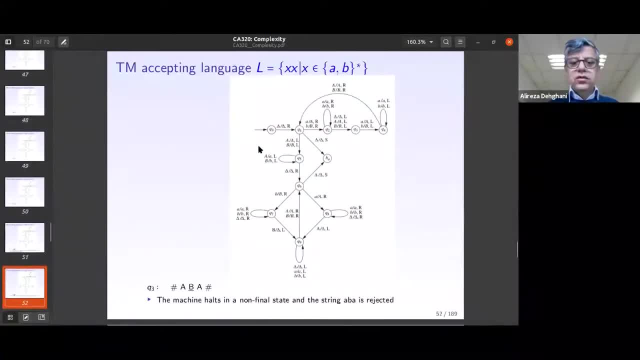 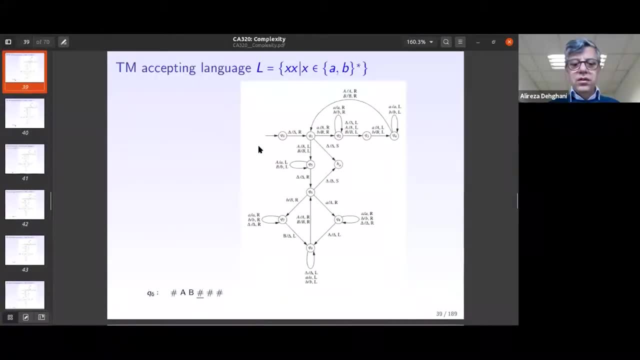 We went through And finally we got to the point which was here and say, OK, machine accept this guy, Machine accept this guy. And also we checked another example which was ABA. We wanted to make sure this machine rejects that. 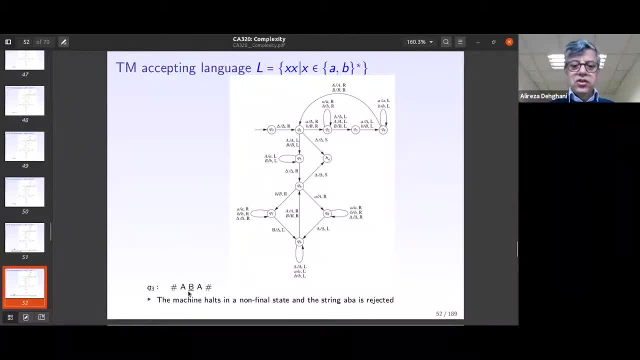 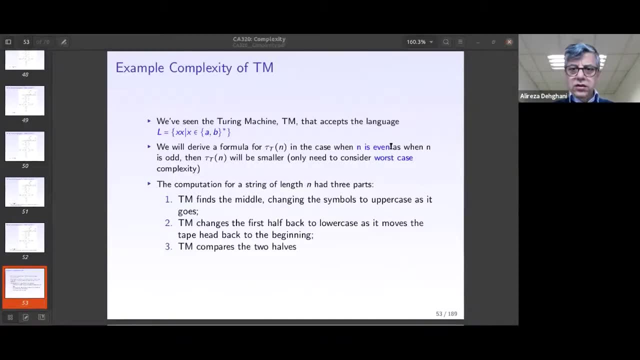 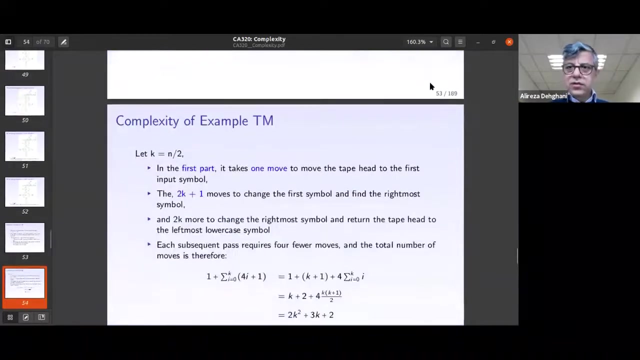 And we examined that and we saw exactly: yes, machine rejects this case. So let's have the chat box in here, Box in here Open in case if there's any question. OK, so Yeah. and then we talk about the complexity of this machine and we say it in terms of complexity. 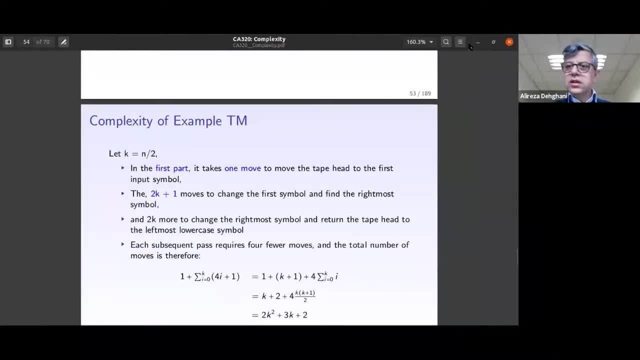 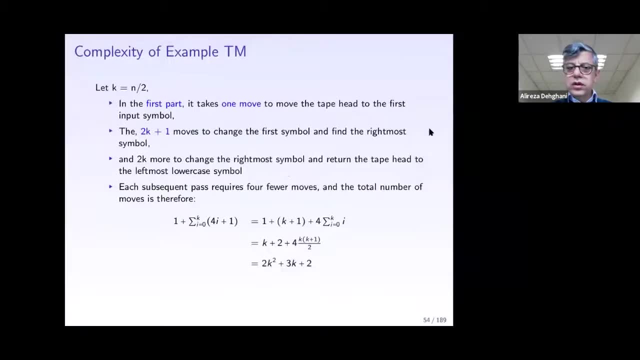 There was somewhere here we could see the presentation in terms of- In terms of present slideshow, Yeah, In terms of This guy. It was much easier to understand And we tried to calculate the complexity of that machine. We say, if you remember, I say the complexity of machine is number of moves you need to take to read specific string and then say OK, if it is accepted or if it is rejected. 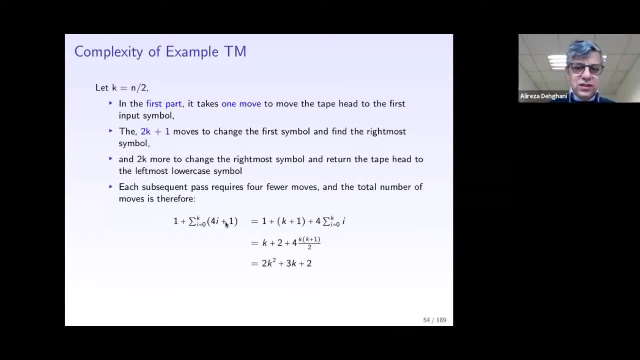 For that specific machine. we calculate different cases. So one case was actually to check if the length of the string is even. I mean, since you want to check if you have something and that thing exactly is repeated at the end- So the half of the string, if it's X, then the whole thing is X, X, reverse. 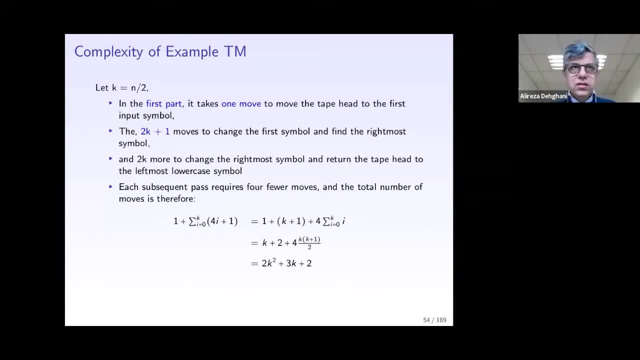 So the length of string should be even. So the first part is to check if it is even the length of string. It takes 2K2 plus 3K plus two moves If the length of the string is N and the half of the length of the string is K. 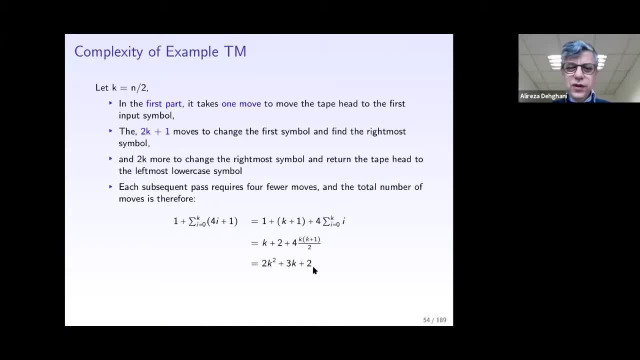 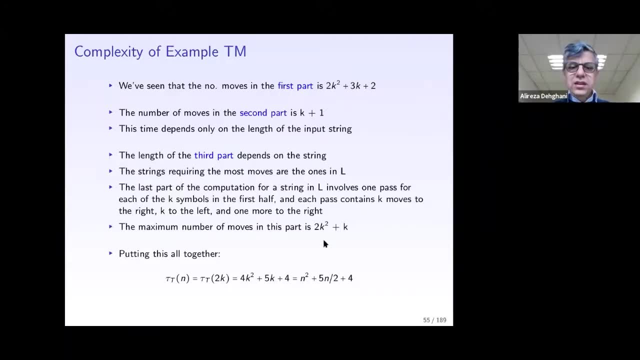 So it takes 2K2 plus 3K plus two moves, And then The second part takes this number of moves And then the last part takes something like that And then if you put all things together, sum of all things together, we will get to N2 plus 5N over. 2 plus 4 is the time complexity of that machine to work on that specific string. 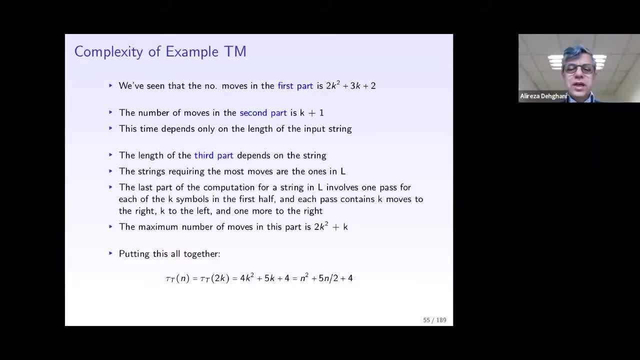 And say: if it is rejected, I accept that. For example, if the length of this thing is six, then you need number of units. You see, the number of moves you need to do is six square plus five, six over two plus two. 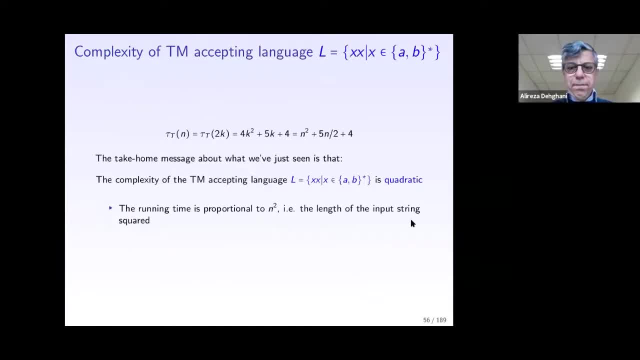 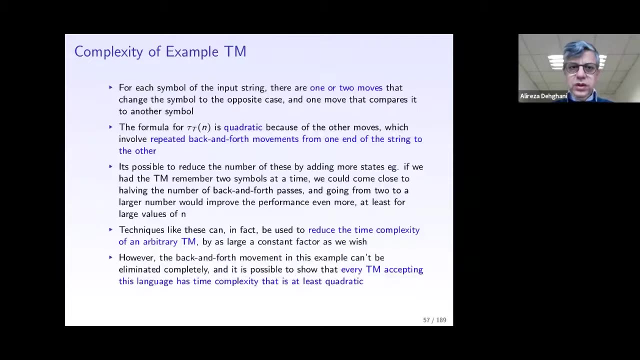 But in general, usually we get rid of the the rest of the stuff, and also only we consider them to. the running time is proportional to N2.. The length of the input string is squared. So then We talked about the complexity. We said, OK, the complexity of the machine is quadratic in this case, because it depends. 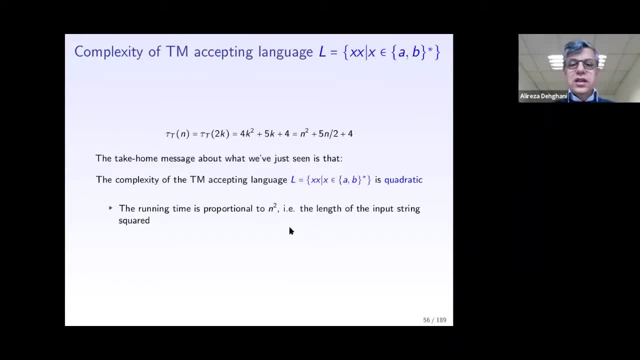 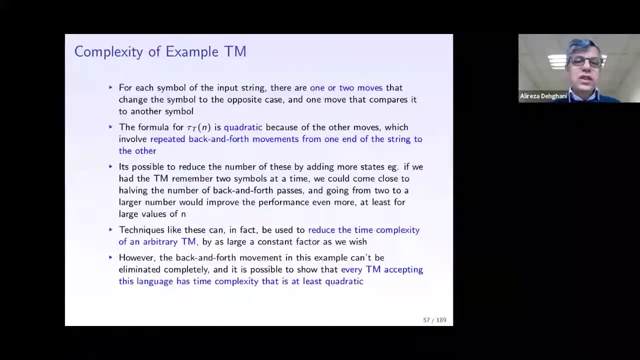 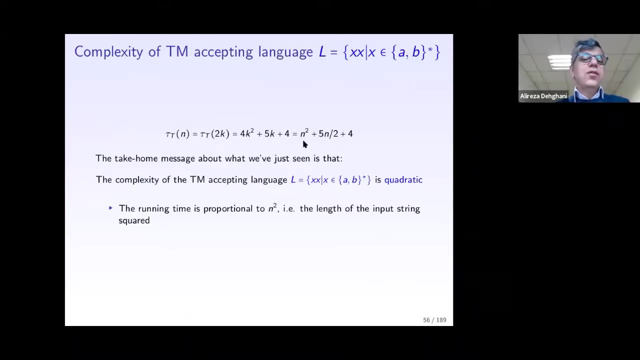 It's proportional to a quadratic statement kind of. And then we got to this point We said it's not a good idea to say, OK, if the number of, for example, the complexity of this specific machine is number of moves it needs. is like that for a specific N. 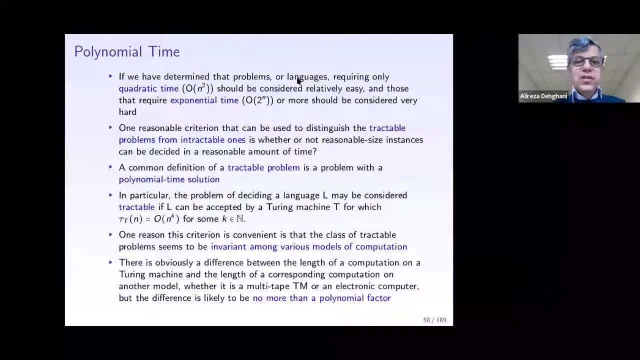 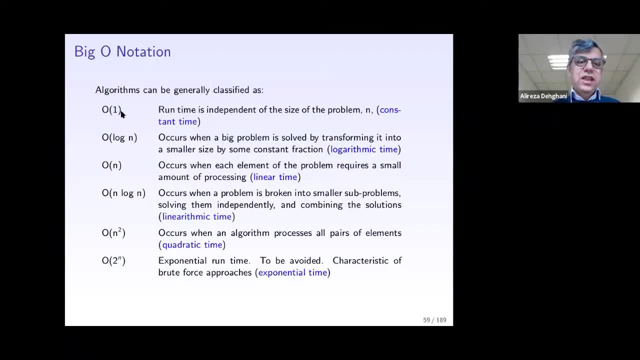 You can calculate it. It's better instead to say Based on N, which is called big O notation, And we discussed the different categories we will have in the O notation. Lastly, that was the simplest and less complex problems. If it is O1, it is. run time is independent of size of the problem. 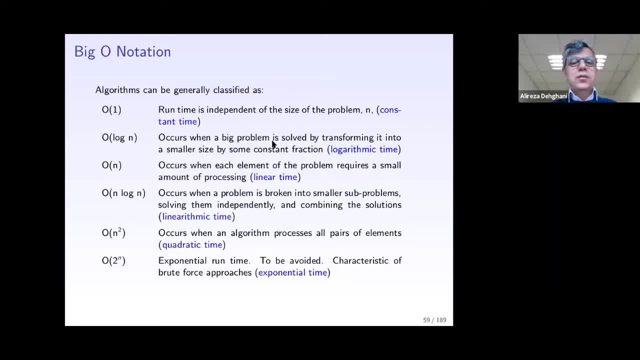 Constant time, like N, occurs when a big problem is solved by transforming it into smaller size. But sometimes, sometimes, it is still not a problem, It is still not complex. The problems that the time complexity of them are: O, log, N, O, N is a linear, like the linear search. 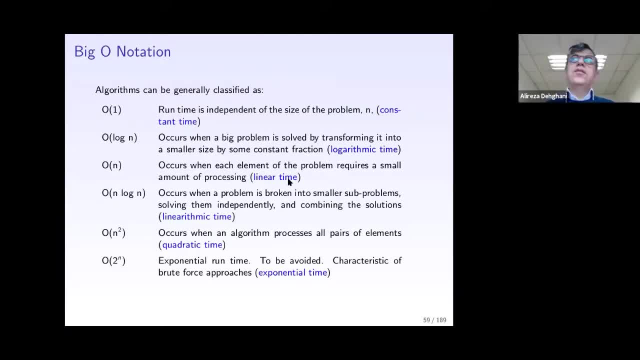 If you want to find something inside the list, If you have that specific thing inside that list, you need to check all the elements one by one, which is linear. So how many times you check the elements of the list is equal to exactly the length of the list. 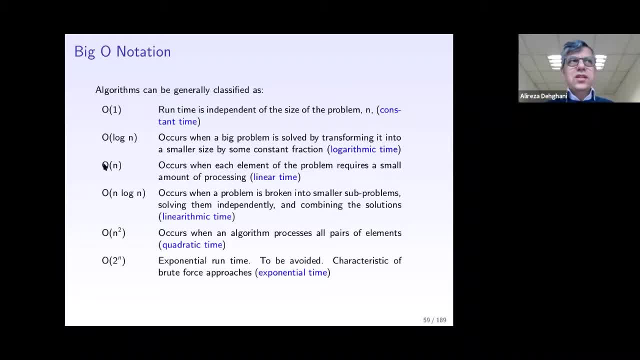 So that's linear kind of the problem, Problems that they're complex. It is linear. The next more a little bit more complex problems are O, N, log, N, Linear time. They are still okay And they are not really complex problem. And the next section are: they are quadratic. 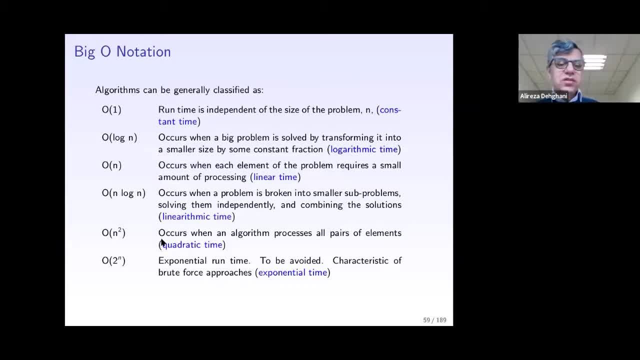 They're called quadratic, like the Turing machine we discussed. Still, they are considered as a solvable problem and not complex problem to some extent. And then the question, And then the craziest type of category of problem in terms of time complexity are O, 2, N. 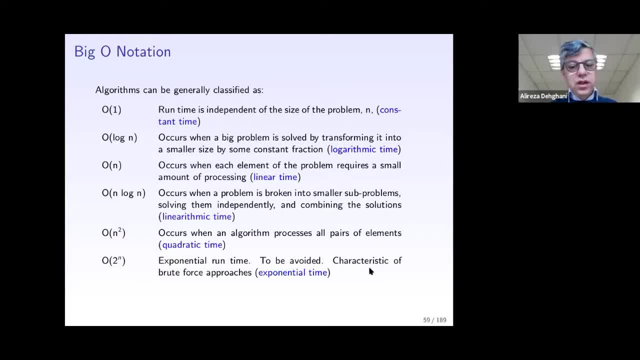 They are exponential runtime to be avoided, Characteristic of brute force approach, exponential time. One of the example of these cases are breaking a cryptography, A crypto, actually Okay. So actually breaking a cipher or solving a cipher could be exponential time Complex. 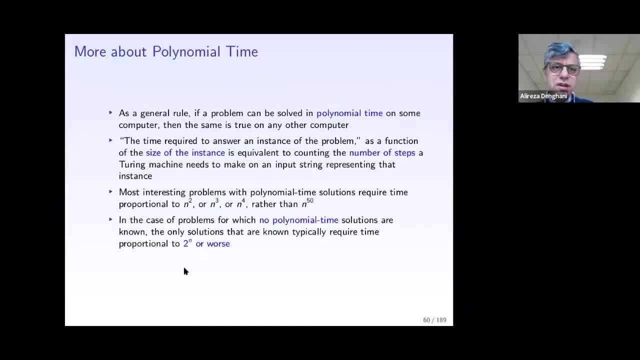 Okay, We got to this point last week. That was a recap last week. But now, as a general rule, if a problem can be solved in polynomial time on some computers, then the same is true on any any other computer. So it's not the matter of the matter of to say, okay, it is solvable on this specific problem, but it is not solvable on other problems. 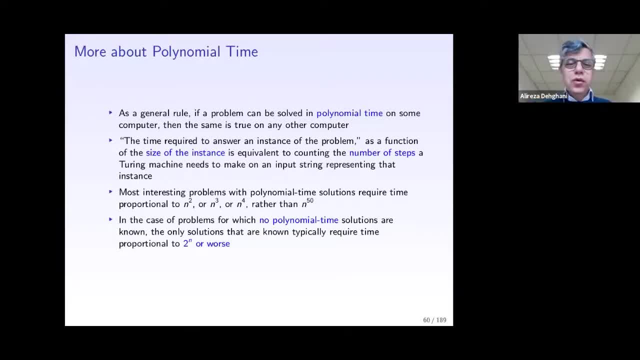 No. If a problem is a polynomial time and it is solvable on other problems, No. If a problem is a polynomial time and it is solvable on a computer, then definitely it is solvable everywhere. If you remember, from the beginning of the semester, we discussed this course is related in two different topics. 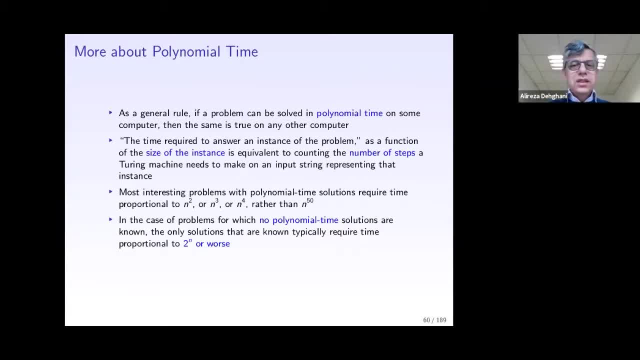 First of all if a problem is solvable or unsolvable, and then if that specific problem that's computable, it's computable, that's computability. And then if it is complex, how complex is solving that problem? If that is computable, solvable. 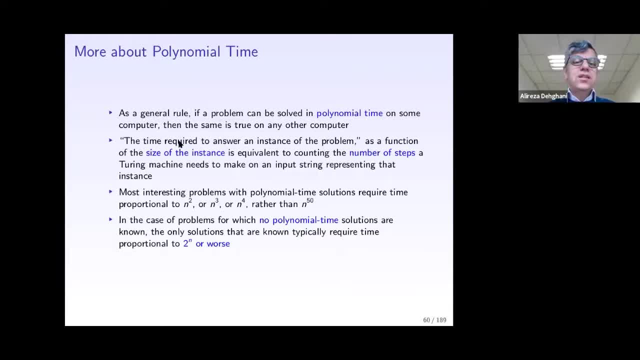 That's the question of how complex is solving that problem. So the time required to answer an instance of the problem, as a function of size of the instance, is equivalent to counting the number of steps. The Turing machine need to make an input string representing that instance. 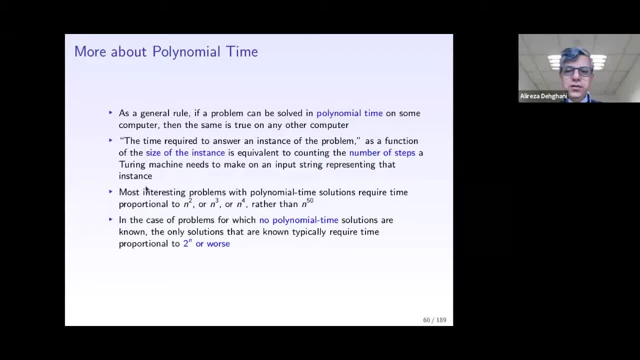 What does it mean? It means we say Turing machine are the basis of computing And we suppose any problem can be dealt with the Turing, using Turing machine. And then so what is the complexity of problem? The problem is the complexity of that machine that can solve that problem. 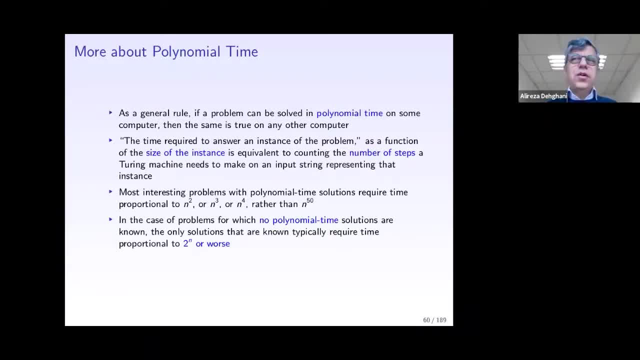 And so that's the complexity of Turing machine that can solve that problem. And what is the complexity of Turing machine? The complexity of Turing machine is the number of steps that Turing machine needs to make an input and an input instance representing the instance. Most interesting problem with polynomial solutions are recall n2.. 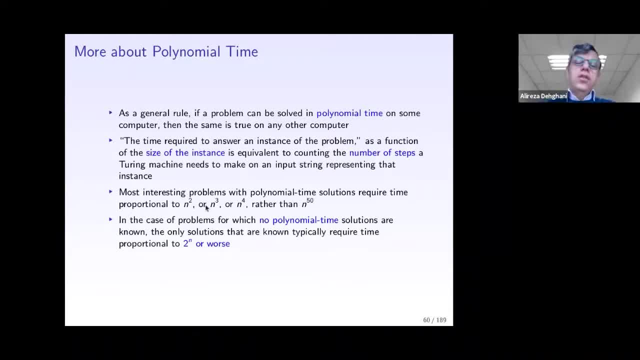 So we say the polynomial problems are the problems. The number of steps that Turing machine solve for each polynomial is n0.. So the problem is the complexity of Turing machine, is the number of steps that Turing machine solves for each polynomial, And so it is not a simple problem. 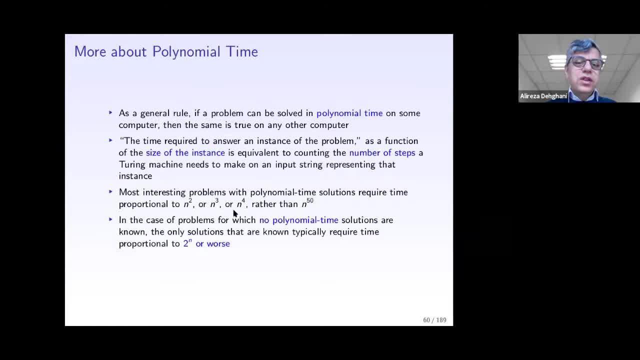 The problem is a complex problem. Now let's talk about the polynomial time solution. The polynomial time solution is a question called real time solution or polynomial-time solution. It is a question that we are going to discuss Why it is a real problem. 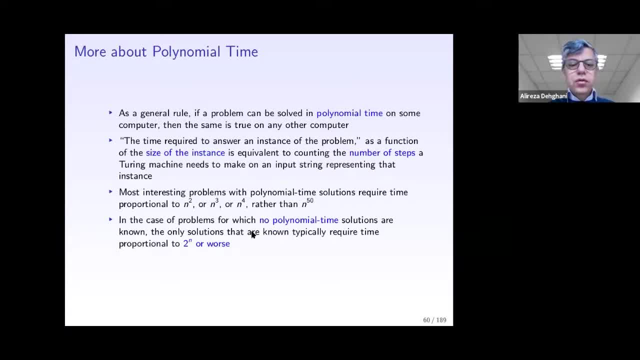 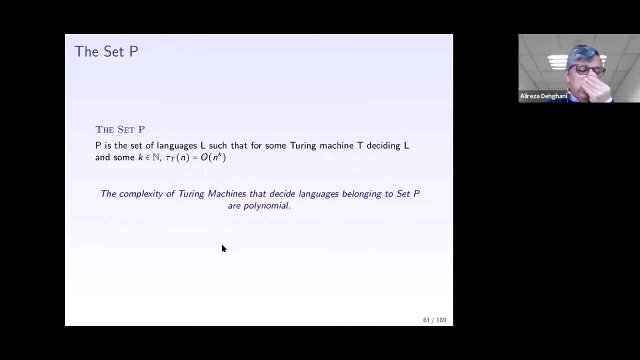 And the real problem is that the polynomial time solution has no polynomial potential, only solution that are typically required or proportional to they are exponential problem. so if you find a problem which is not polynomial or it is non-polynomial time, they are definitely exponential, which are two power, n or even worse than that. okay, based on what we have, we have, we 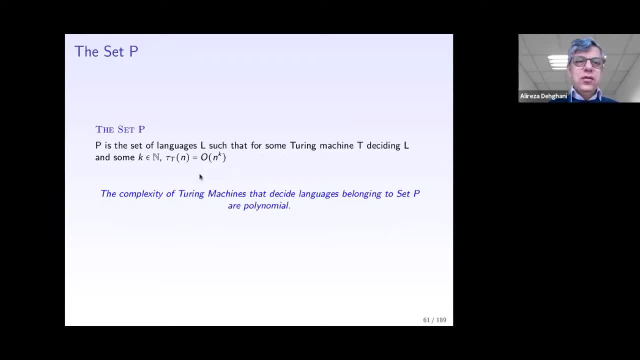 talked about. in terms of time complexity, we can categorize the whole number of problems in two set of p and n p's. okay, the set p problem p is the set of languages, l, such that for some Turing machine t deciding l and some k, the time complexity is polynomial. so p are the problems. 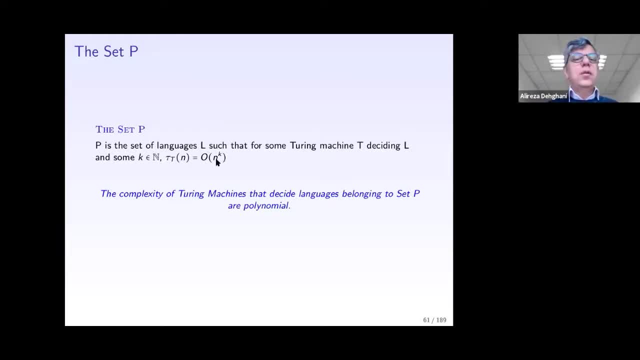 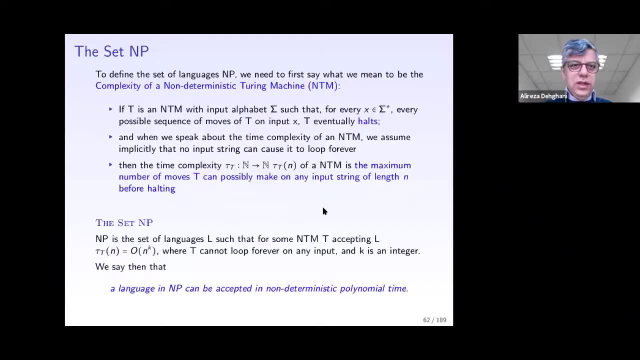 which they time complexity and the Turing machine is polynomial. the complexity of Turing machine that decide languages belong to set. p are polynomial. okay, what is the set of non-polynomial, non-deterministic polynomial? okay, so to define the set of languages, n p, so we have p and n p. okay, for to define the set of. 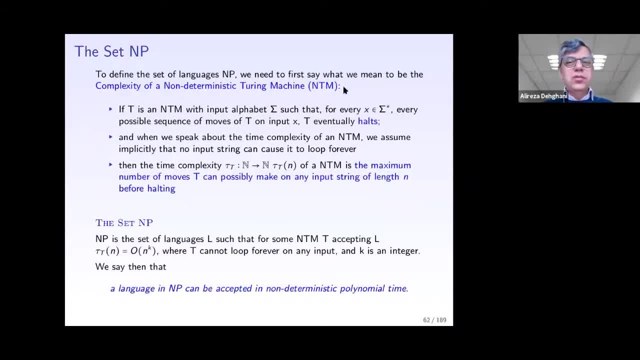 languages n? p. let's have a look at non-deterministic Turing machine first. if Turing machine is, if t is, is a non-deterministic Turing machine, with alphabet sigma such that x belongs to any sigma star, every possible sequence of moves of t on input x, t eventually halts. imagine t is a. 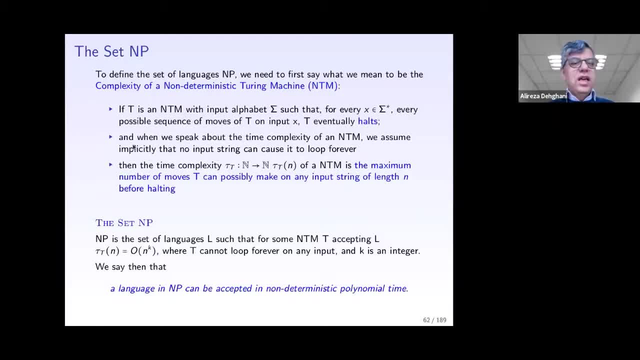 non-deterministic Turing machine which halts. finally, and when we speak out the time complexity of ntm, we assume implicitly that no input string can cause the loop forever. okay, so we just we are excluding these things. first of all, we assume machine will halt at some stage. you remember, in Turing machine we had definitely the situation that. 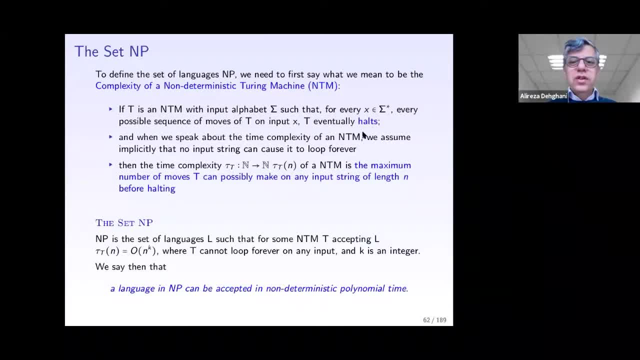 machine can loop forever and it won't halt. okay, so the machine should halt and it there is no input string can cause the loop forever. okay, so the machine should halt and it there is no input string can cause it to loop forever, then the time complexity of that non-deterministic Touring Machine is the 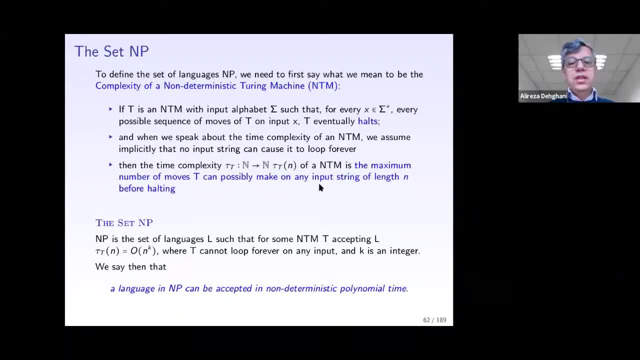 maximum number of moves we discuss that can possibly make any inputs belonging to it then. so that's the definition actually we discussed also. then what is the set? np is the set of languages that for some ntm turing machine accepting L, the time complexity is polynomial where 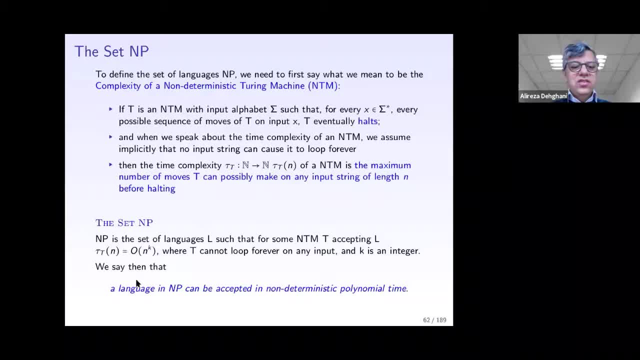 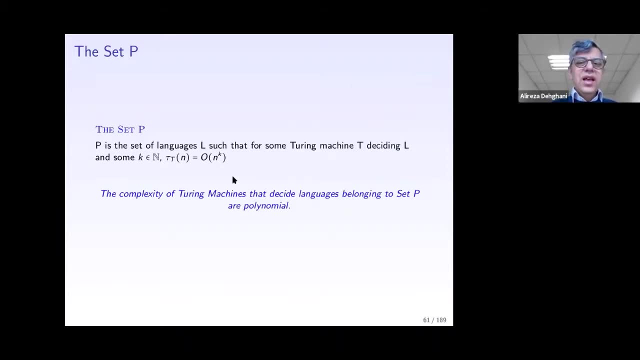 t cannot loop forever and k is an integer. we say then the language is: np can be accepted in non-deterministic polynomial time. so, as you can see, there is not that many differences, that much differences between p and np. p is a language which is uh, which has a time, complexity of. 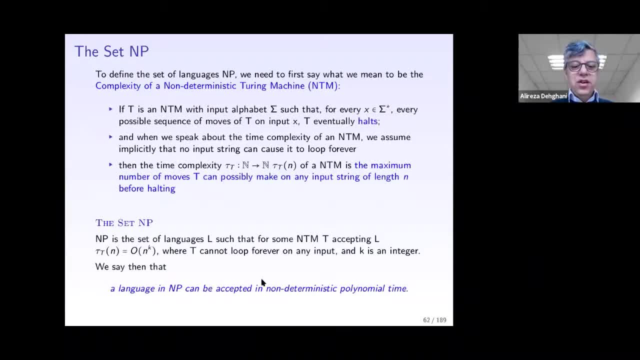 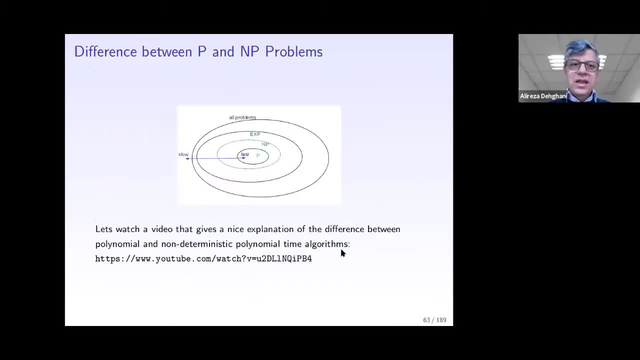 polynomial also to np is kind of a language which is which can be accepted by non-deterministic polynomial time. but that's the matter of another specific things. if you look at the thing, probably we can discuss it here in a better way. so if that's the whole problem, all problems, the big 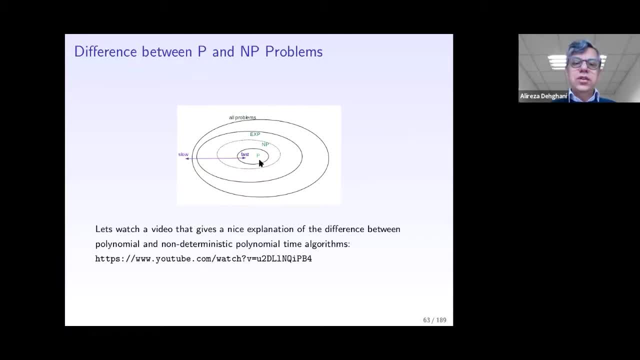 all okay, and then we can categorize them into different classes. we have classes of p, we have classes of np, exponential, and all problems, as you can see, p and np, all of them are polynomial, they are not exponential, so they still are polynomial problem. what does it mean? it means probably they should be solvable. okay, but that's. 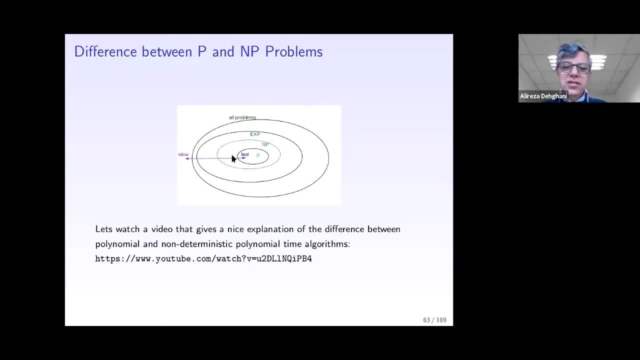 the matter of how complex is the solution. is it easy or is it hard to be solved? if it is even very, very complicated and complex, they are exponential and at some stage they are probably unsolvable. and there are probably other problems more complex than the exponential problems which 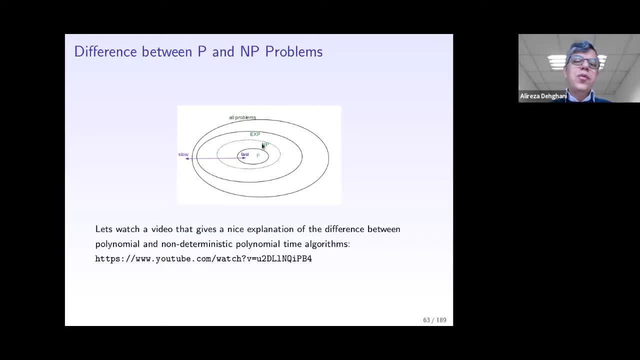 sit inside this area, into the other side of the problem. so that's the problem and then we can say that all problems. but like we discussed in here, we have the p and np problems. for the p problem they are a easier problem that you can solve them. for the np problem, still they are non. 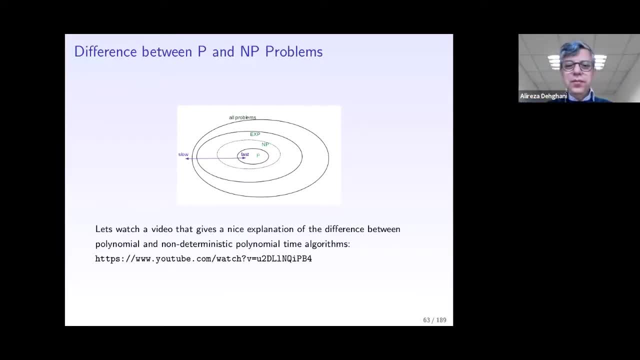 they are polynomial problem, polynomial time problem, which they are harder the problem. so in terms of time, complexity, you see, whatever we get inside toward the p problems, the p set, they are faster to solve and whenever we go toward the outside of these guys you can see they are smaller to solve. there's a video which has been shared in: 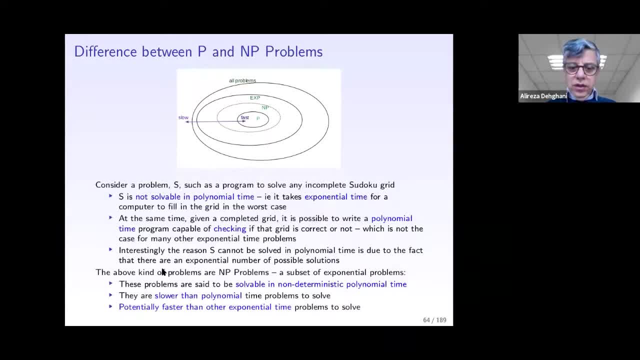 here. you can watch it later yourself. but i will share more interesting videos with you later at the class, after the class, inside the in the course webpage, which are really interesting. so consider problem s such as a problem to solve. any incomplete pseudocode grid s is non-solved, not solvable in. 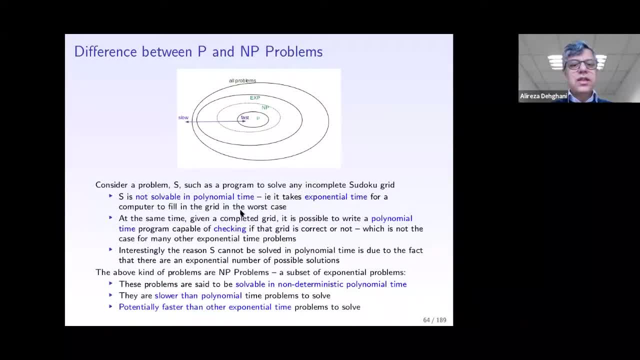 polynomial time, ie it takes exponential time for a calculator to build a grid at the worst case. at the same time, given a complicated grid, it is possible to write a polynomial time program checking if the answer is correct or not. interestingly, the reason s cannot be solved. 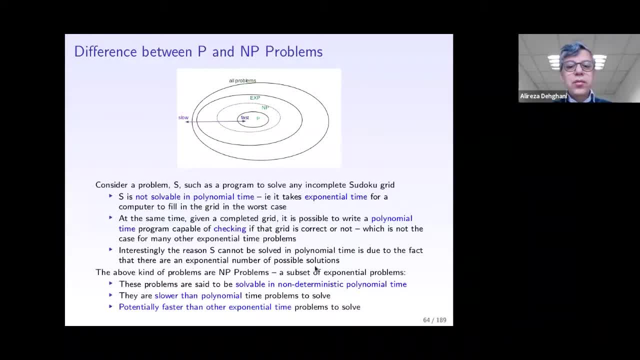 in polynomial time is due to the fact that there are unexplainable number of possible solutions. the above kind of problems are NP problems, a subset of exponential problems. these problems are set to solvable in non-deterministic polynomial time. they are slower than polynomial time. there is a little. 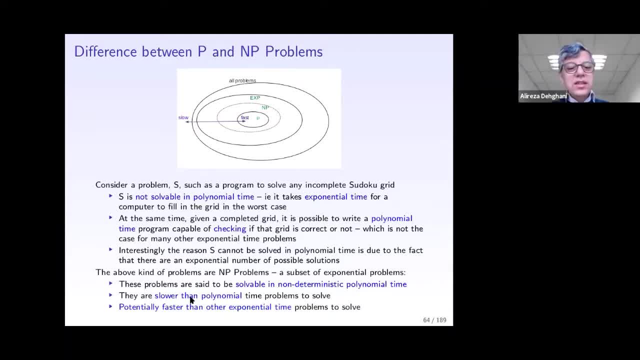 bit different in here: non-deterministic polynomial time and deterministic polynomial time okay, potentially faster than other exponential okay. so that's very interesting thing and cases are in here. so we said we have the most interestingly for us there are. we have the np and p problems. np is a subset of p problems. p problems they 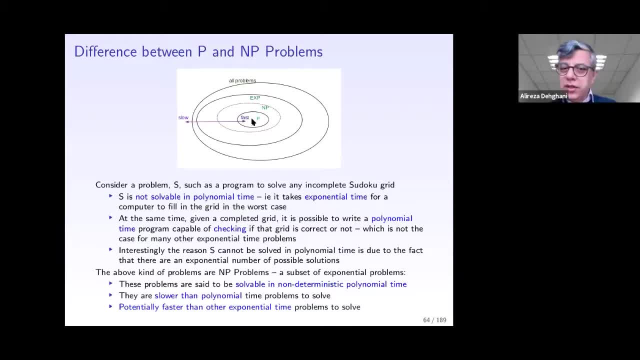 are time complexity or polynomial time complexity. np are non-deterministic polynomial time complexity and exponential or exponential time complexity. okay, they are really complicated and complex problems. pseudocode, jigsaw- they are two examples of the cases- and even chess they are example of cases we sit in exponential and non-polynomial problems. okay, so what is the main? 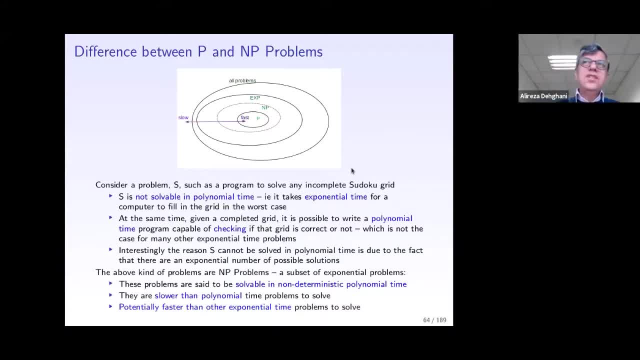 question, which i think there is an question or no. so what is the the main thing actually we can categorize? let me share with you another screen, the problem we have in here. if you remember, in linux, when we switch to another date, it doesn't show that. so i need to reshare the things. 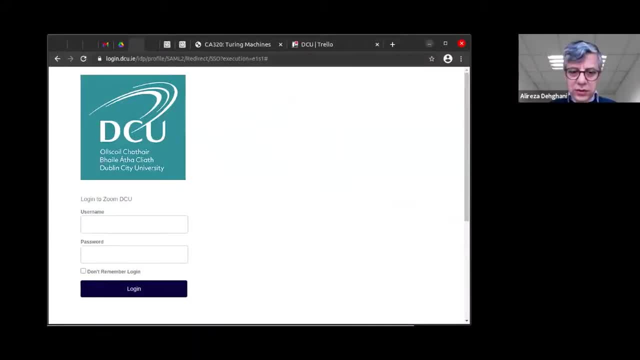 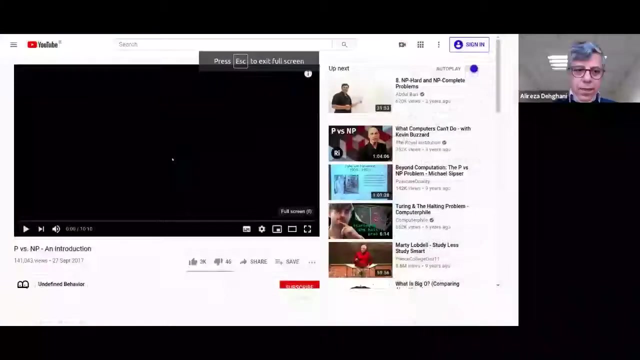 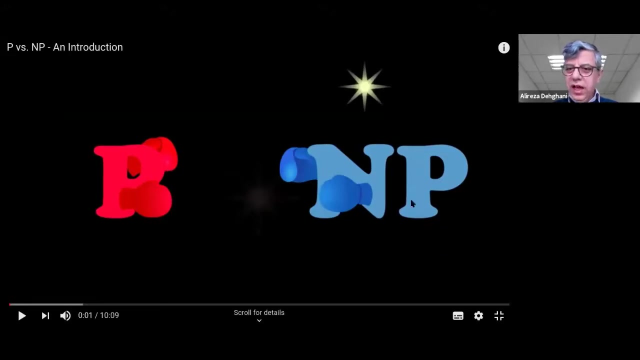 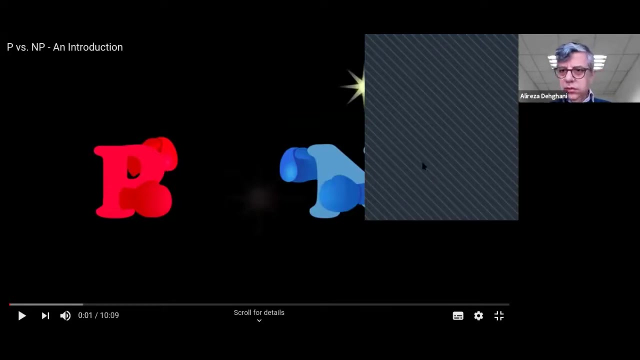 that's not the case. let me share another string in here. is that the case? no, let me exceed the full screen and in here. okay, so let me share a new screen with you. you should be able to see what this screen. okay, can you see the the YouTube page I have shared and see the YouTube share page? yes, thank you very much. 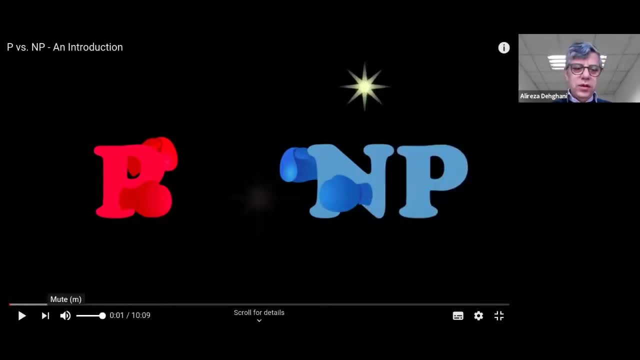 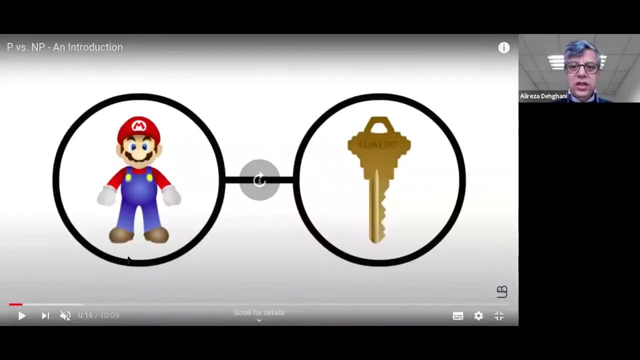 okay, so that's a very interesting video. I don't want to play the whole video in here. probably I will fix on some some slides and I'll talk about that, so I will share this video later with you, if you see. so that's the matter of if we really talk about the NP problems or people. 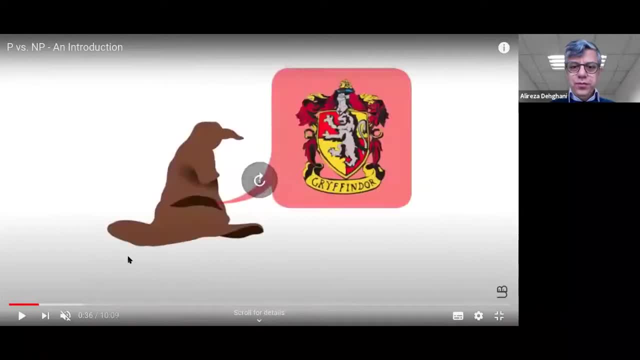 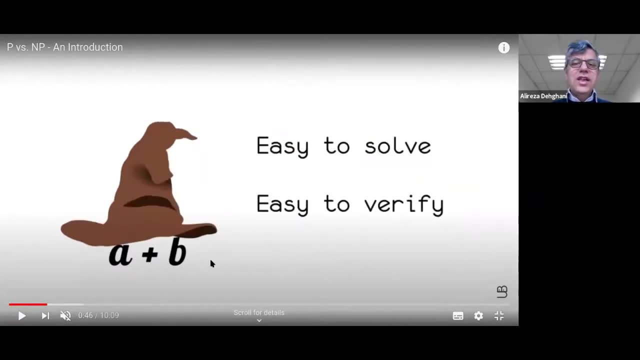 problems. we are talking about distance, okay. so imagine we have some problems like: what is the summation of a and b? they are really easy problems, okay. they are easily easy to solve and easy to verify. that's the key criteria of understanding the difference between the P and NP problem, okay. 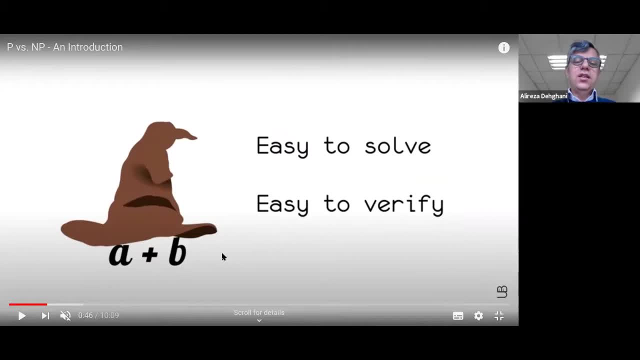 so P problems are category of problem which they are easy to solve and also they are easy to verify. can you understand the difference: easy to solve and easy to verify. easy to solve, it is completely clear. can you solve this problem for me, yes, how complicated, how complex is it is easy. can you let? 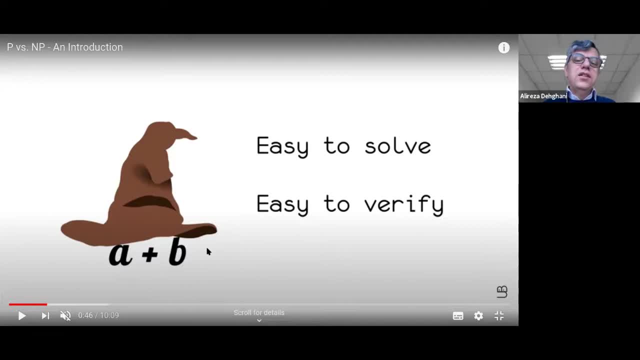 me know what is the summation of a and b? yes, I know, and that's easy to solve. and what about the verification? if I have the solution of the problem, can I say if that's correct solution for that problem? that's the verification. okay, so is it easy to verify that? 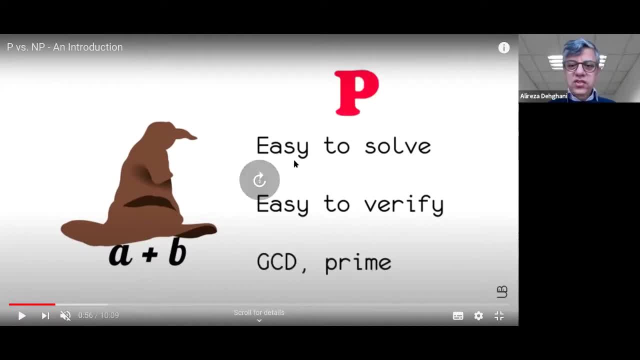 the P problem is: most things are easy- solving the problem and verifying the solution. okay, for example, if the number is prime, it is easy to solve. is it easy to say if the number we have said prime is prime? yes, it is so easy to verify the answer. okay, so these are the set of P problems. 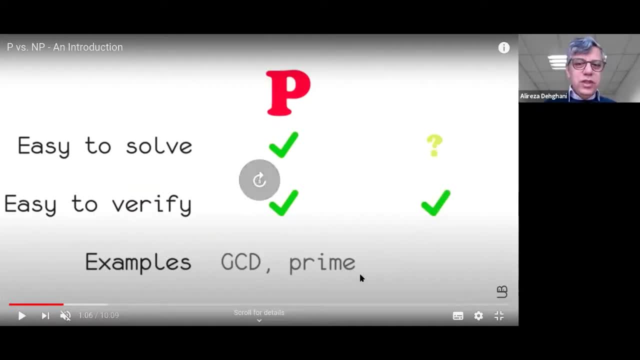 so they are easy to solve and they are easy to verify. but we have another class of problems which they are not usually easy to solve. they may be maybe see this. they don't say they are, they are not easy. it may be easy or may not be. 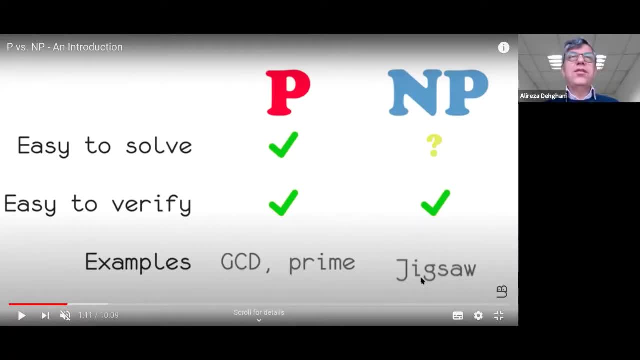 easy to solve, but they are easy to verify, like the jigsaw. if we have a jigsaw and if we ask you if it is possible to solve this problem, to complete this jigsaw, you might say, ah, it's not, I don't know, it's not easy to solve it because that's up to the jigsaw the size of. 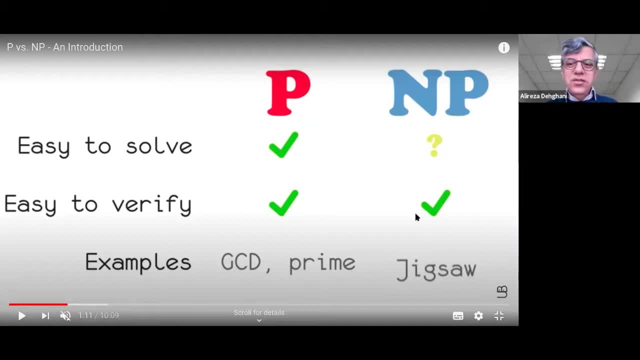 the jigsaw and the things. well, is this easy to verify? if the solution is okay, if someone has completed the jigsaw already for you, can you say, is that a correct solution to that? yes, exactly. you can check all the pieces one by one to see if they sit correctly beside each other and complete the. 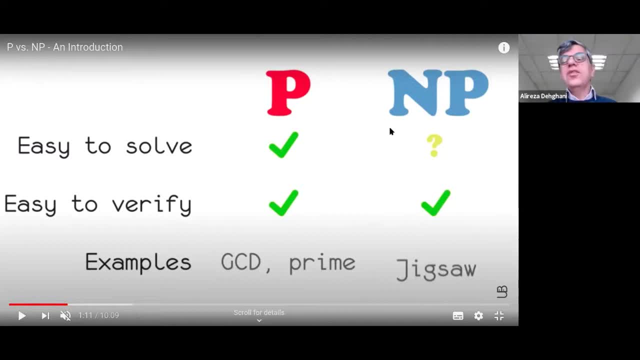 image we are expecting, so the verification is easy. so they are kind of the NP problem. I think that's the best description of P versus NP problem I have found. I will share this video with you later. you can watch it yourself. so, like I said, that would be. 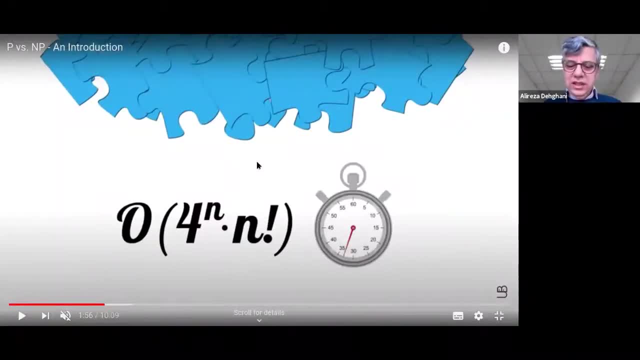 the case. exactly as you can see, it tries to say the same thing in here. so for the jigsaw, for example, as you can see, the time complexity is something like that. it is really hard to solve this problem, although nowadays we have computers that solve the problem where they say the problem. 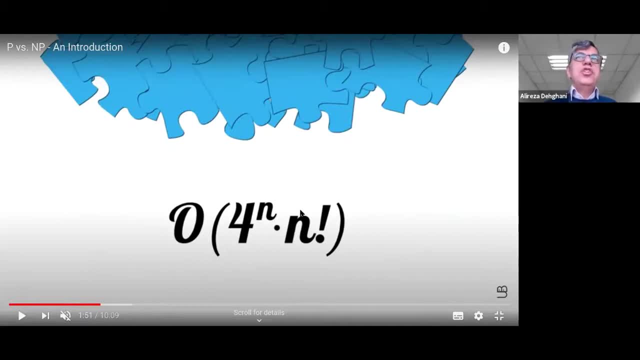 is NP or a problem is exponential in terms of time complexity. it doesn't mean necessarily it is unsolvable. no, it means it is hard to solve. they have lots of NP problem which they are not solved yet, but lots of them they have been solved. so that's the matter of how hard it is the NP it's. 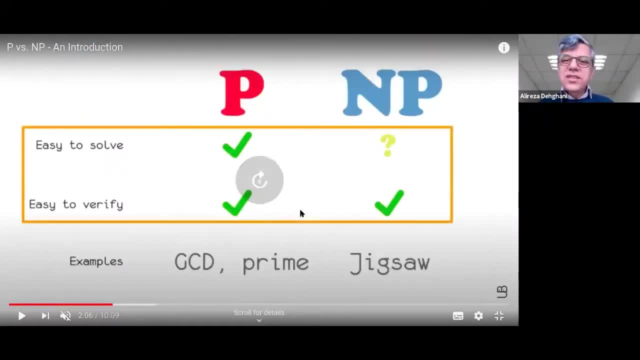 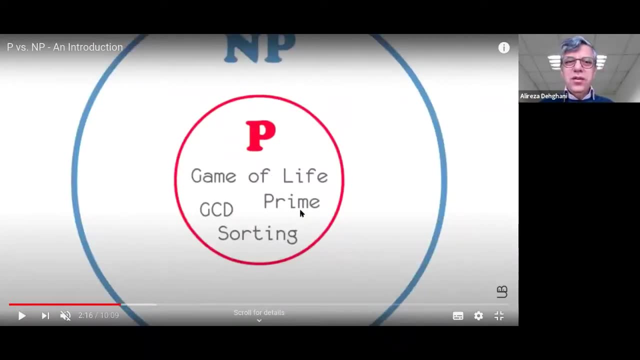 not a matter of it is not possible to solve. so, as you can see, that's exactly the same case. it is not easy to solve, but it is easy to verify. so that's the matter of comparison. P is a subset of NP. P problems are the problems which are easy to solve. 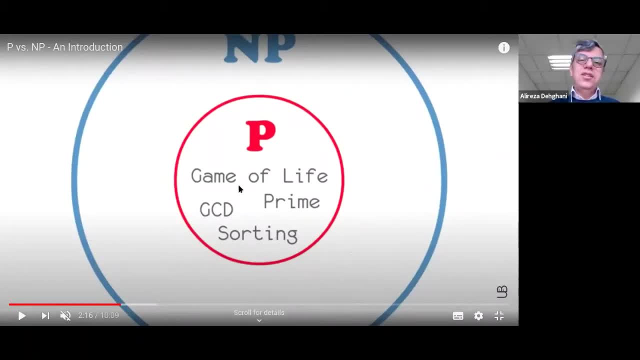 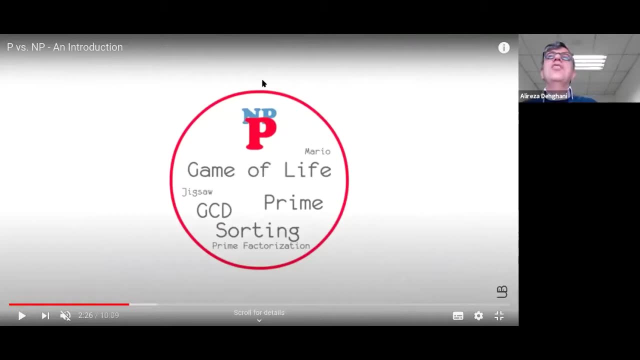 easy to be verified: entry problems, not easy to solve but easy to verify. so they are subset of NP and so that's one of the open problems. there are seven millionaire problems in physics and mathematics. they are the problems. they have not been solved yet and they have been seven. 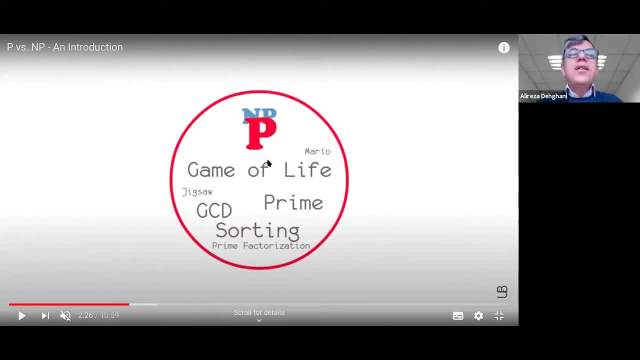 if you can solve any of them, you will want a million dollar price. so we can start from today to solve one of those problems. one of those problems have been solved already by Riemann, one of the scientists. okay, and still we have six problem unsolved one. 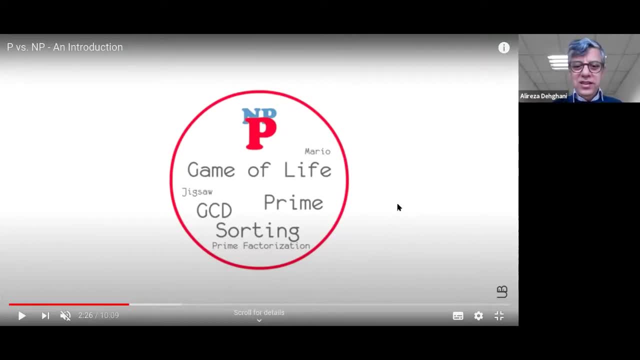 of those problems, unsolved problems, which scientists are interested to be solved, and the world by itself, let's say the is interested to be solved, is the if P is equal to NP problem. if P is equal to NP problem, what could be the outcome? what would be the outcome? the P problem in the P problem, you say. 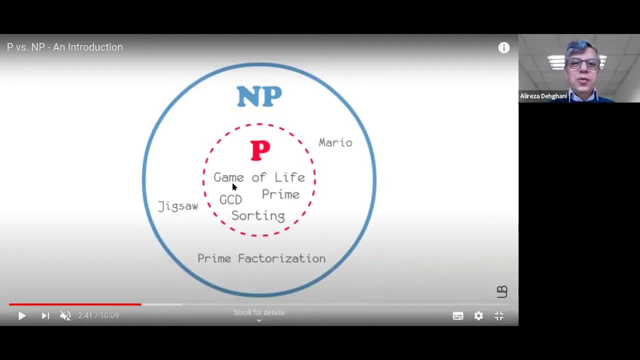 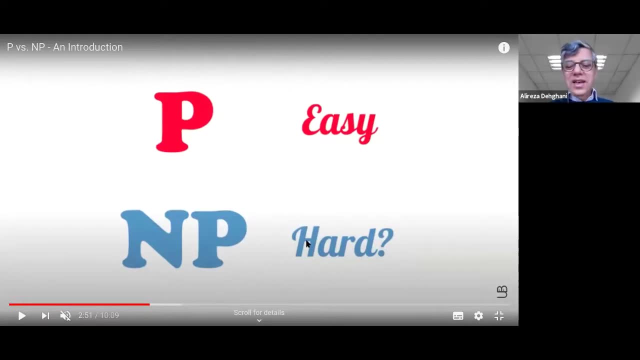 is it to solve, yes? is it to verify, yes, for the entry problem you say: is it to solve? no? it is hard, probably. is it to verify, yes, if they say P set and NP set are the same, then what would happen? if you say P and NP set they are the same, what would happen then? 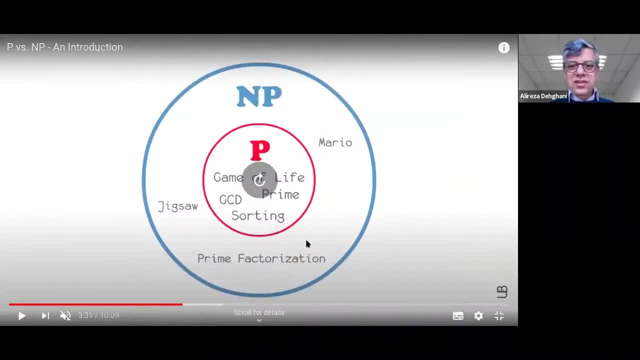 let me see I don't want to go to these three things. let's just stay in here. if you say P and NP problem are the same, then that means lots of problems which are hard to solve at the moment can be solved easily. it doesn't mean the proving N is equal to NP will give the solution to all. 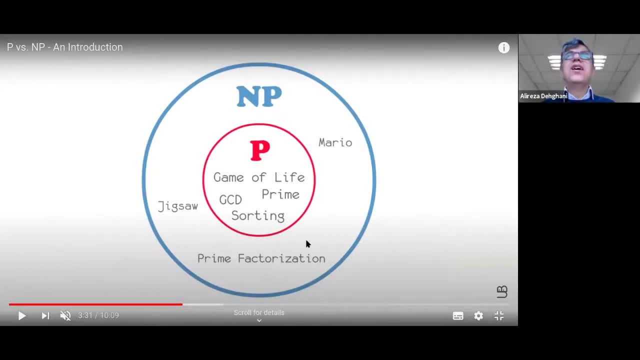 those hard problems to us? no, it's not the case. what it means? we can justify that if a problem if P and NP are the same, if P and NP are the same, then that means a problem which is hard to solve, which is easy to verify then would be easy to solve. that's all. so one of the crazy NP problem. 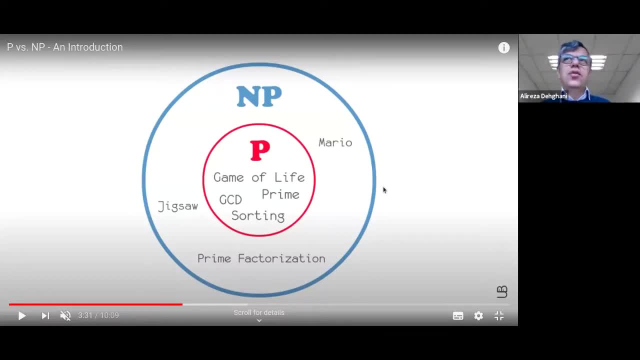 playing the music. we have lots of musicians in the world, right? so, like Mozart, he knew how to compose the music to be beautiful. that was a problem. what is the problem? is it possible to compose music which everyone loves it in the world or it is very favorite? that's a. 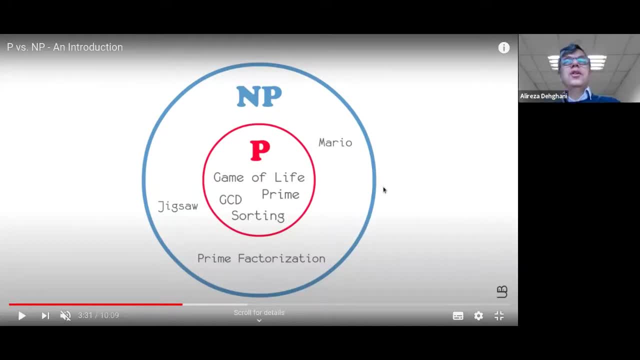 hard question to ask. that's a hard problem to solve. but what about the verification? is the music that Mozart composed is beautiful? you can listen to the music and say, yeah, that's beautiful music. so that's one of the NP problems. so if we can verify the P and NP problems are the same, then 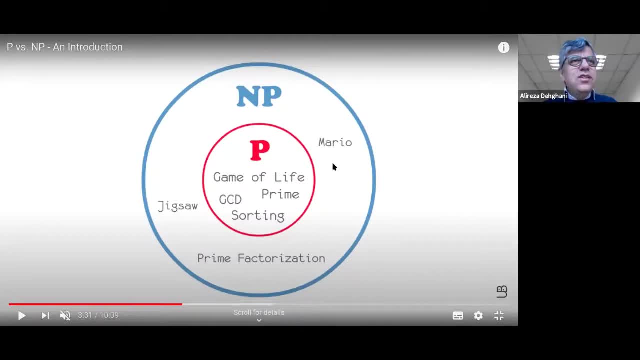 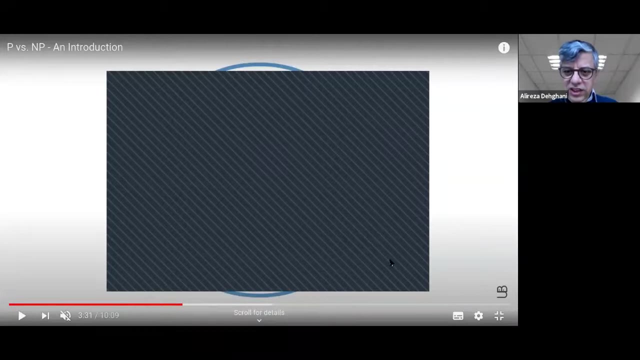 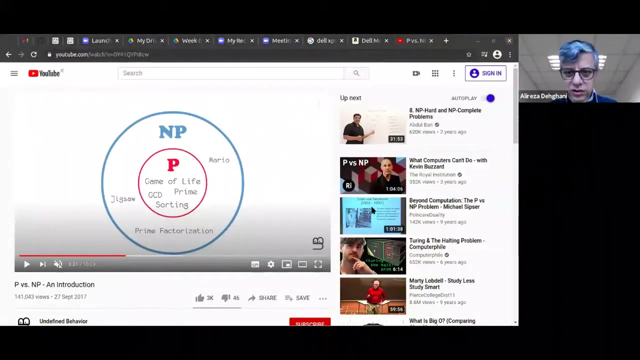 what does it mean? it means easily we can generate musician like Mozart. right, so that's the interesting part. okay, so that's the problem of P and NP. let's back to the presentation. let's back to the presentation. I will share another screen. hopefully you should be able my presentation, not the Chrome, not the complexity in here- share. 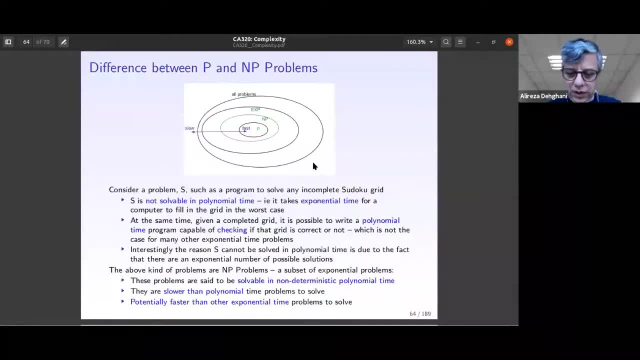 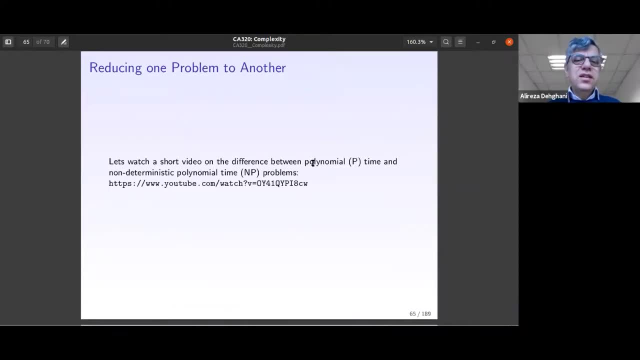 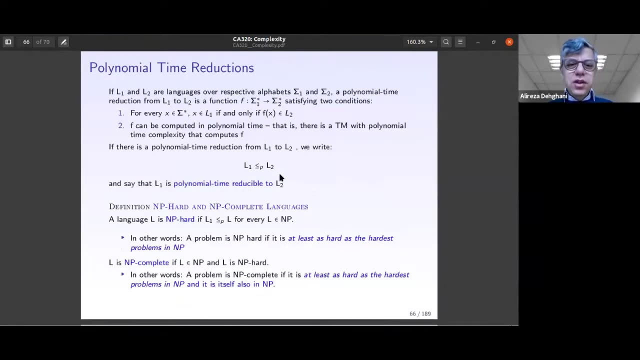 okay, so that's the matter of P versus NP problems. okay so, and reducing one problem to another is the story of how we can reduce an entry problem to a pre-problem to P prop polynomial time reduction. so if L1 and L2 are languages over respective 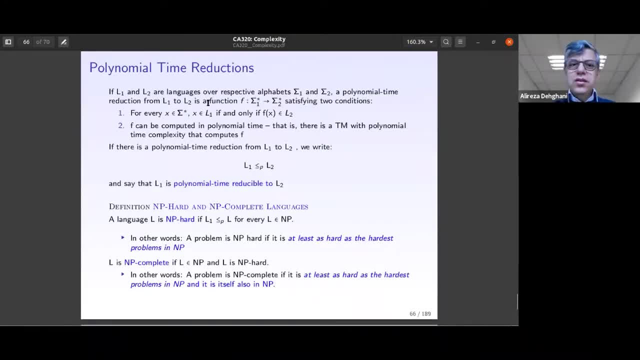 alphabets: Sigma 1 and 6, Sigma 2, a polynomial time reduction from L1 to L2, is a function which, for every X belong to Sigma to L1, if, and only if fx belong to L2. we discussed that somehow previously, so that's the matter of. 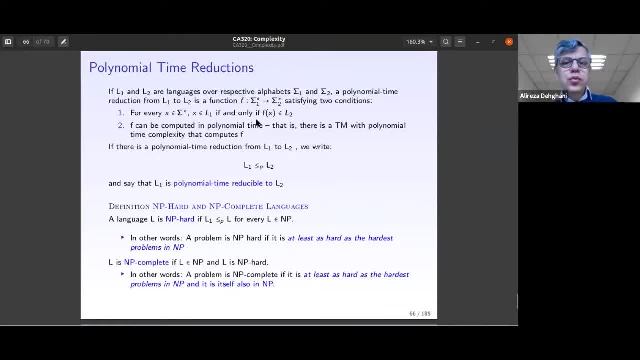 how we can reduce that polynomial time problem to simpler problem. okay, so to say, if we can find another languages which is similar to the first language and it is easier, so that's the we will say. L1 is a polynomial time reducible to L2 definition. 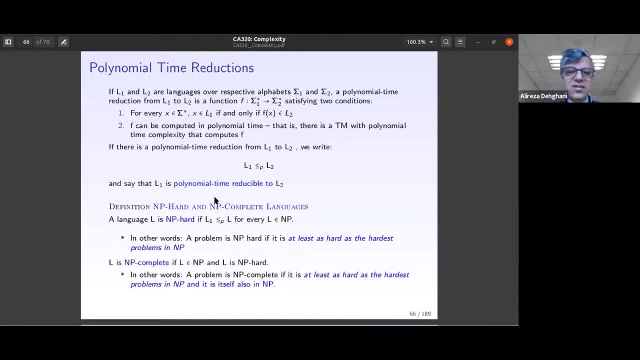 of okay. so in NP set we have NP hard and NP complete languages. the language L is NP hard if L1, uh less than equal L2 for every L belong to NP. in other words, the problem and the problem is NP hard if it is at least as hard as positive, as hard as the problem in the end. so and the problem 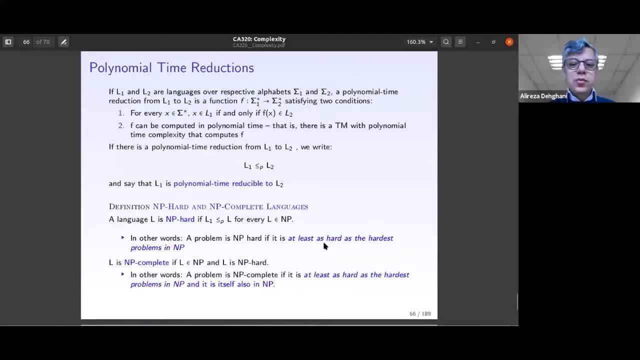 NP is called NP-hard if it is kind of the hardest problem in the NP set, And NP-complete if a problem is NP-complete if it is at least as hard as the hardest problem in NP and it is itself also in NP, So that in other words the hardest problem inside NP called NP-complete. 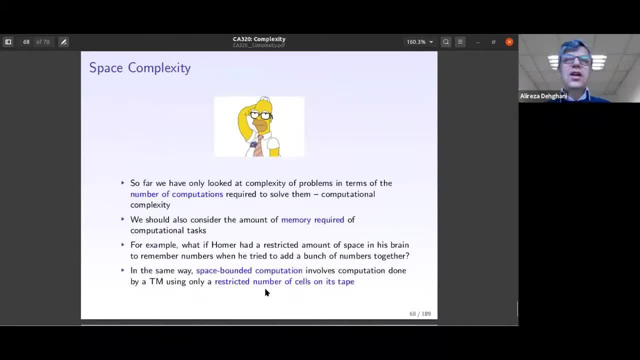 They are the hardest problem inside the NP-complete. Okay, so that was the matter of complexity. When we talk about the complexity of an algorithm or a problem, so we are talking about two different things. The first thing is the time complexity, which we discussed by far, how much time it takes to solve this problem. 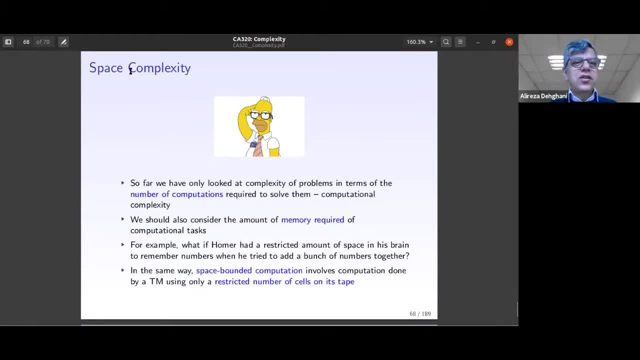 That's the time. complexity. But we are facing with another version of the complexity, which is space complexity. okay, So far we have only looked at the complexity of problem in terms of the number of computations. So far, we have only looked at the complexity of problem in terms of the number of computations required to solve them: computational complexity: 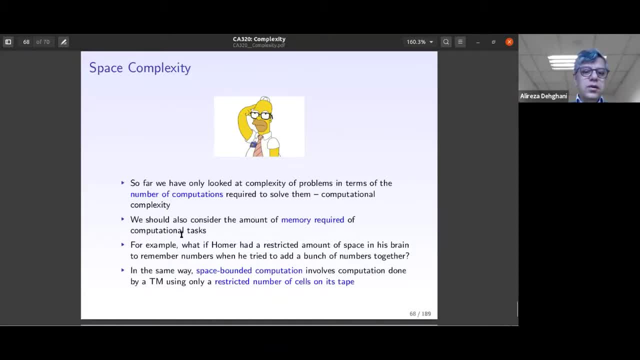 We also consider the amount of memory required of computational tasks. For example, what if Homer had the restricted amount of space in his brain to remember numbers when he tried to add a bunch of numbers together? In the same way, a space-bounded computation involves computation done by a Turing machine using only a restricted number of cell and its tape. 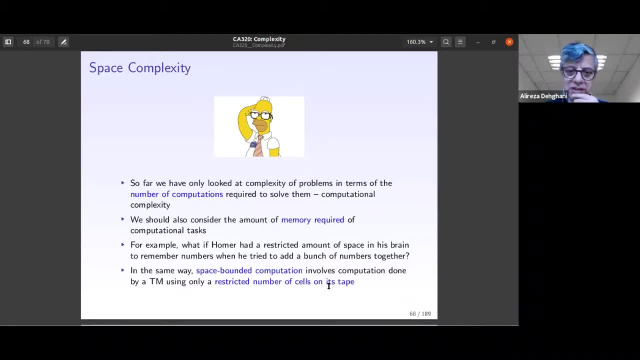 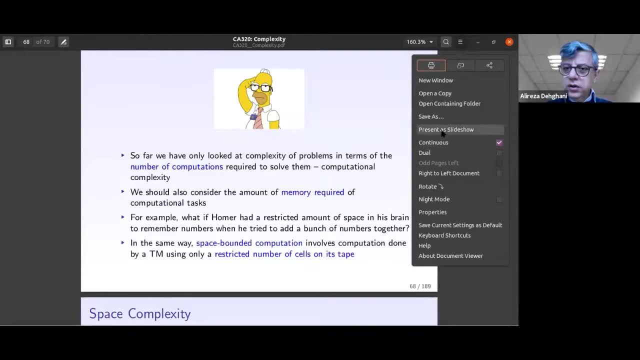 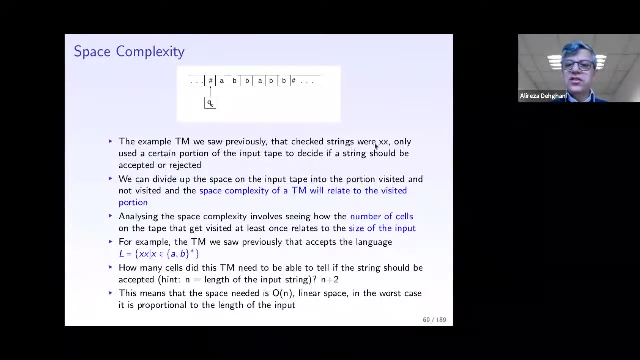 So see, We have kind of the space complexity all the time. It was full page. Okay. so the example Turing machine we saw previously that checked the string where xx only uses certain portion of input tape to decide if the string should be accepted or rejected. 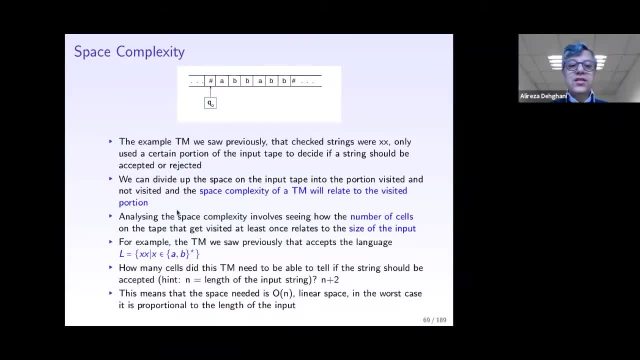 We can divide up the space of the input tape into portion visited and not visited And the space complexity of Turing machine will be related to the visited portion. okay, So for Turing machine, you remember the tape was infinite. the length of the tape. 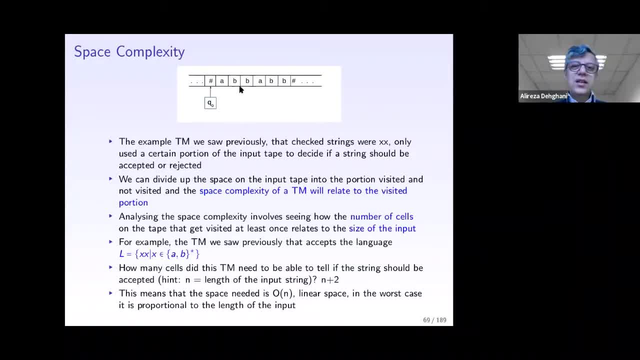 You could write and read, You could move right and move left. okay, That was the definition of Turing machine. So what is the space complexity of a specific problem? It is the portion of the tape actually you visit while you want to accept or reject that specific string. 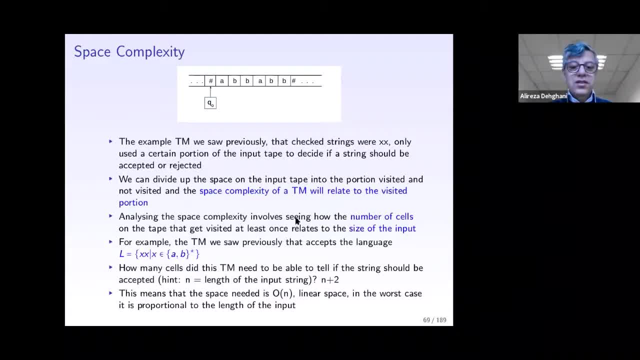 So definitely if it is so. analyzing the space complexity involves seeing how the number of cells on the tape that you get visited at least once relates to the size of the input. for example, for this specific we saw previously accept the language. how many cells did this Turing machine need to be able? 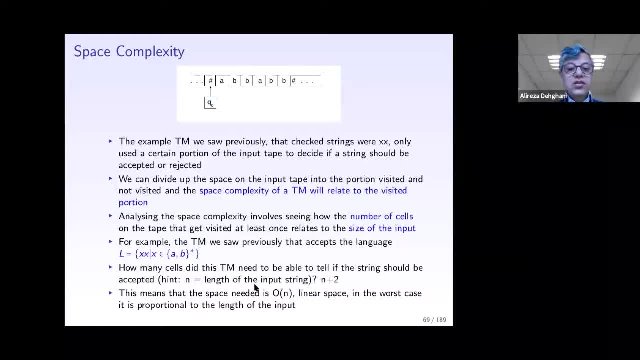 to tell if this thing should be accepted, and was the length of the string. so n plus two was the number of cells we needed why? because we needed to start from a blank in the beginning and then move to the string, and then we needed to get to the point. we see all the symbols of the input. 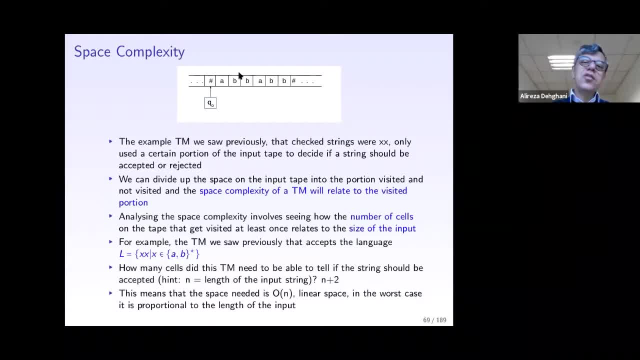 string and get to a blank and then reverse back. you remember a lot of forward, backward movement. we did to accept this specific string. so the number of cells we need to visit at least once on the tape is n plus two. so this means that the space needed is 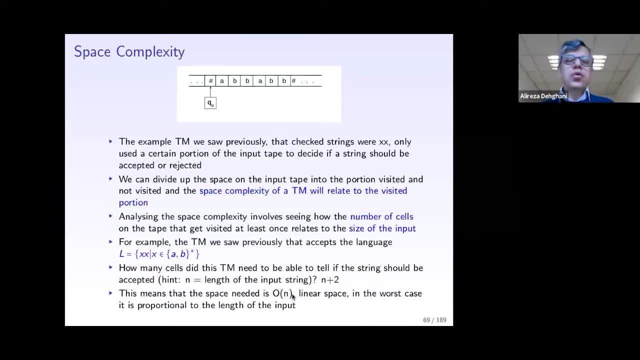 O and linear. you remember, in terms of big, big O notation. if it is linearly dependent on the size of the input string, it is linear O n. so the space complexity of this Turing machine is then O. n is the worst case. it is proportional to the length of the input right. 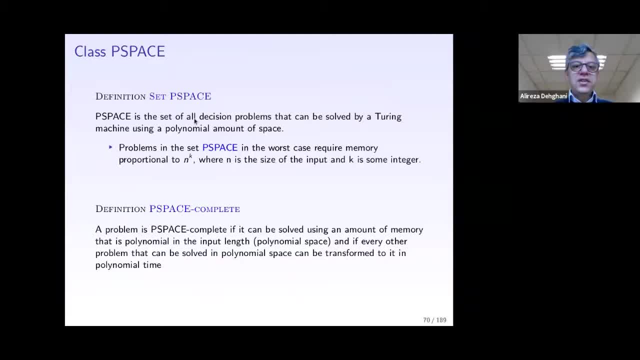 so set PSP. PSP is set of all decision problem that can be solved by Turing machine using polynomial amount of polynomial amount of space. that's exactly the same categorization we had for the time complexity, you remember the P and NP. so the set PS space is the set which the space complexity is polynomial. 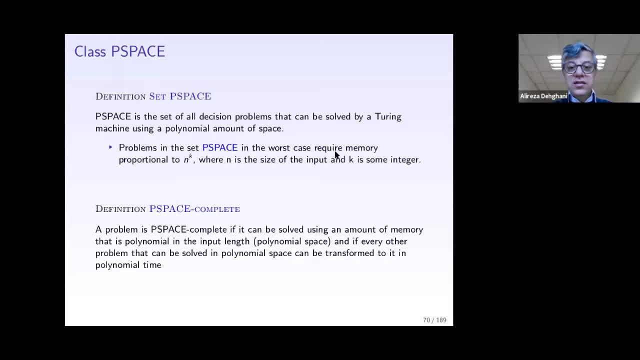 problems in the set. PS space is the worst case in the worst case. requires proportional to NK, where N is the size of the input problem. PS space complete. a problem is PS space complete if it can be solved using amount of memory that is polynomial in the input length and if every other problem that can. 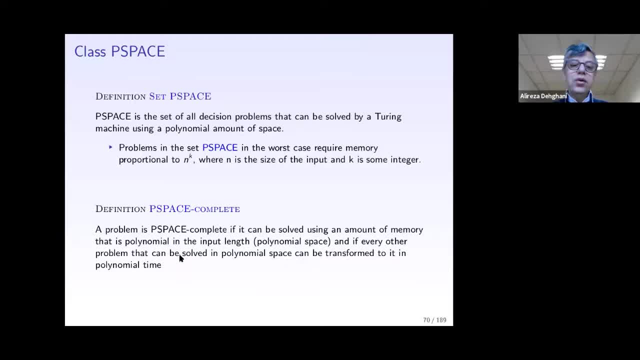 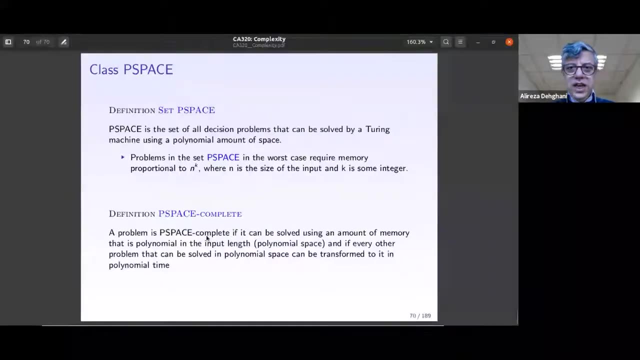 be solved in polynomial. space can be transformed to it in a polynomial. so that's again the same categorization of the time. complexity, the space complexity is kind of the hardest problem in the PS- space problems, okay, but still it is the same, okay. so we have finished. 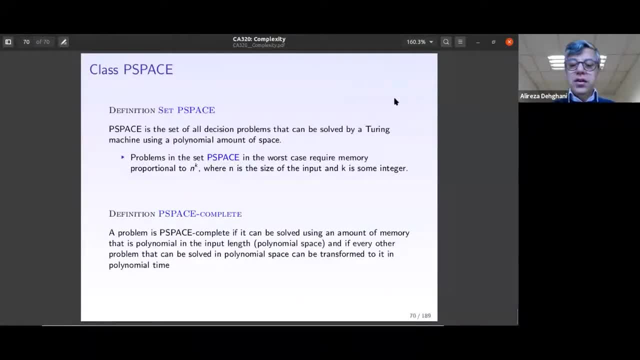 by far the complexity problem. we have another topic to discuss for the rest of today and I have a common data, for let me select this video and divide it. how many of our Ministry as one parallel? hey, what's the order of the order? what's the order of a 100 year term? 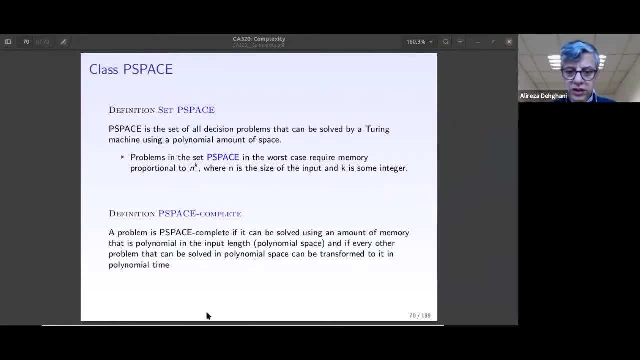 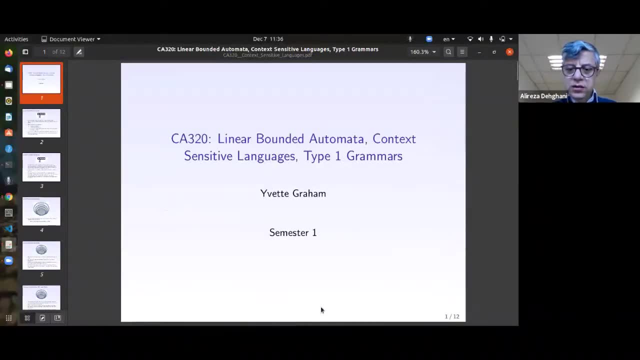 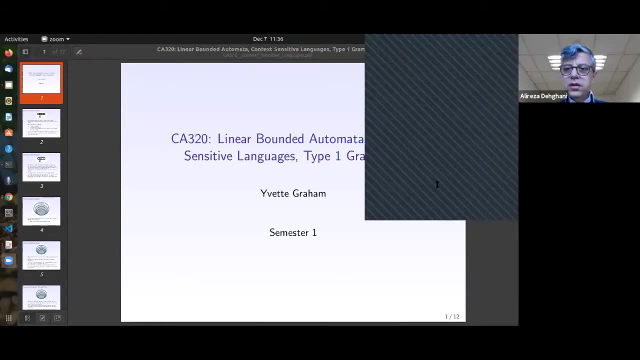 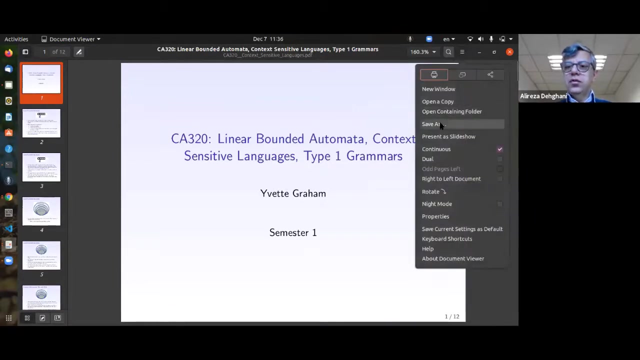 so this is the first a sets of. this is the from 0 to a 100 year term. ok, so let us just rewrite the variable ok s screen, which is the linear bounded automata. can you see the linear bounded automata? yeah, very good, thank you very much. okay, so the last. that's the last, the final topic we want to discuss. 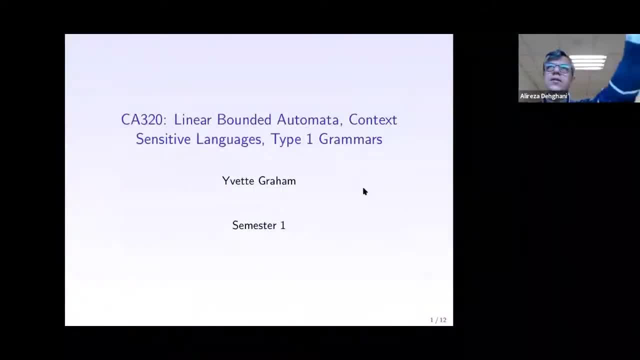 in this course, in this module. so by far, if you remember the chomsky hierarchy we started with, you know we had four different circles inside each other. the smallest one, the inner one, was the type grammar, type three, which was the regular grammar, regular languages, and the machine was the. 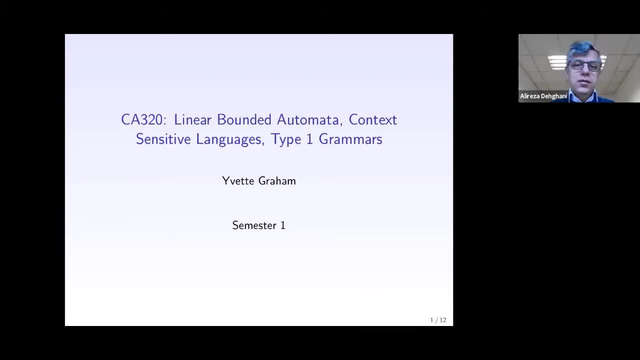 finite state automata, deterministic and non-deterministic. and then we came up one level, the bigger subset, which was grammar type two, it was the pushdown automata, it was text context- sorry, context, free languages. and then another bigger one, the two, bigger one actually if we have the chomsky. 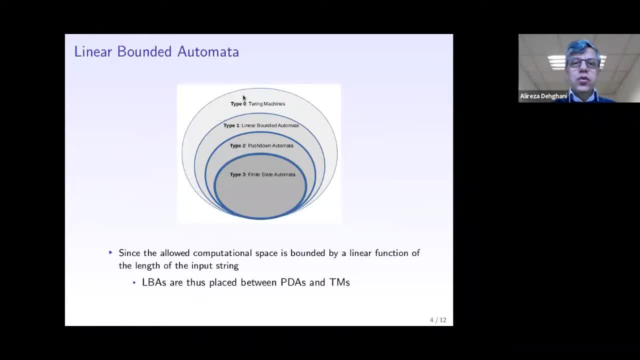 hierarchy here. yeah, and we had another, bigger one, which was the type zero languages, it was context free and it was turing machine. if you remember, in here we are going to talk about another set of languages and machines and automata, which is called linear bounded automata. 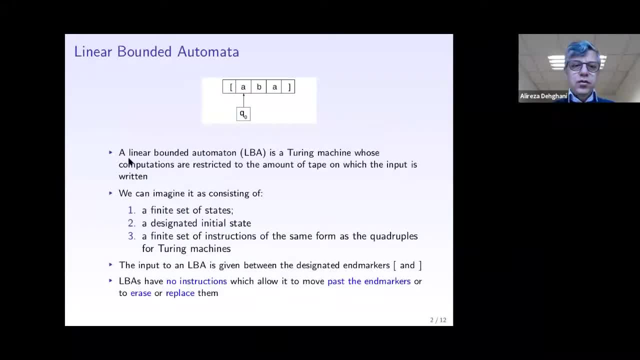 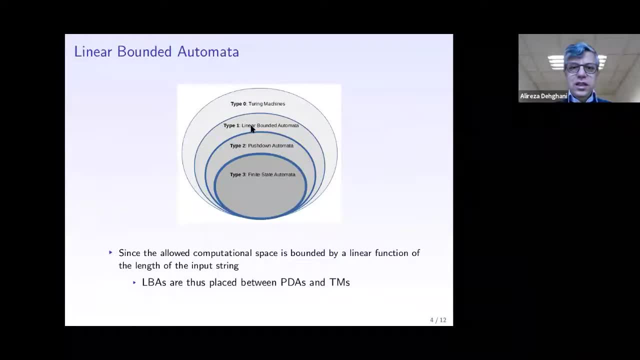 in this module. that's the last topic we want to talk about. so a linear bounded automata is a turing machine subset. as you remember, in here linear bounded automata is a subset of turing machine, so it should be possible to be defined in the case of turing machine there. so 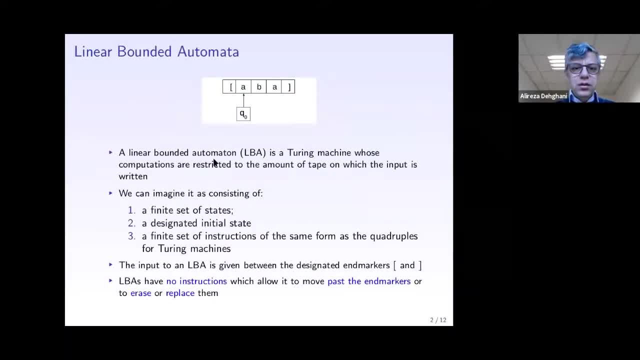 the first slide. okay, a linear bounded automata lva is a turing machine whose computations are restricted to the amount of tape on which input is written. so, as you can see, it is exactly the same as the turing machine. we have the tape, but the difference with the turing machine is that 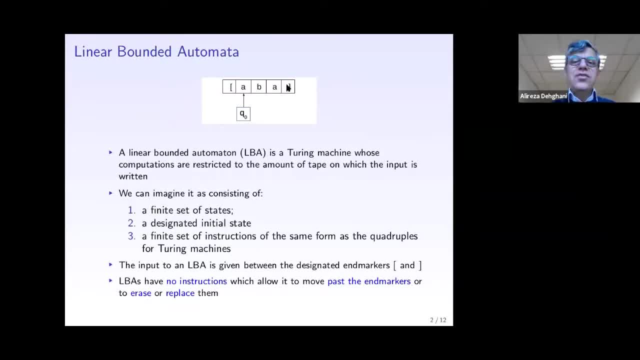 the amount of the tape we can use is the same as the turing machine, so we can use the tape and read and write is fixed. it is not like we can move infinitely to the left. we can move infinitely to the right and we have some symbols, which is starting symbol and ending symbol in here. okay, 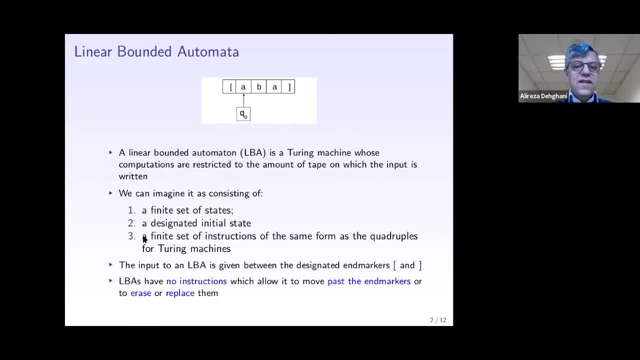 so that's the definition. we have a finite set of states, a designated initial state, as usual, a finite set of instruction, as usual, same form as the quadrat of the quad and quadruple of four turing machines. so we have the same sort of definition of the Turing machine for the instruction we have initial. 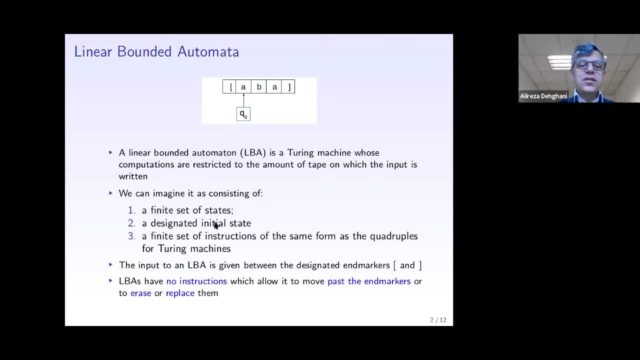 state. we have a finite set of states, number of finite set of the state. everything is the same. so that means we can move right, we can move left, we can write, we can read. they are the same as a Turing machine for LBA, but the input to 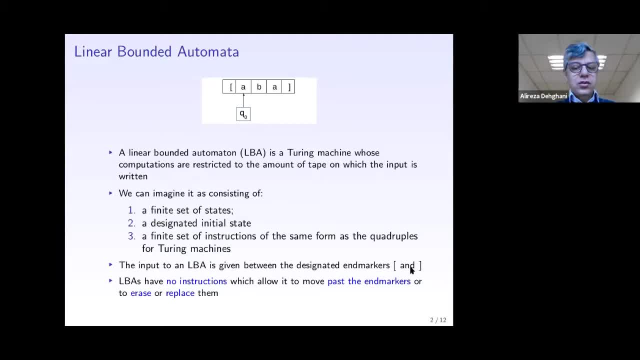 an LBA is given between the designated end marks. okay, you have the beginning starting in and once and the end and once. okay, LBA have no instruction which allows it to the move past the end mark or erase or replace. so it's. there is no instruction at all. this is not allowed to move toward the left of the end marks. 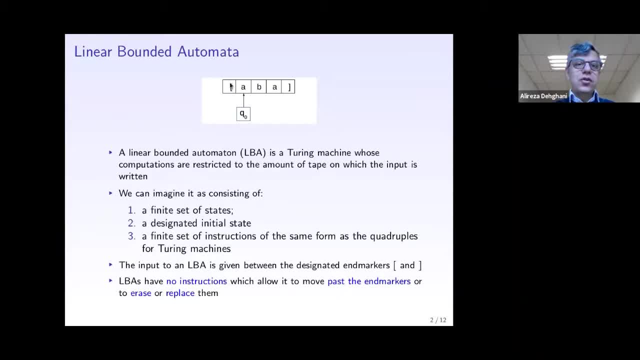 and also erase them or replace them with something. so they are there all the time and you can move exactly in this area and that's the reason why it is called bounded. why? but why it is called linear. you can move exactly in this area and that's the reason why it is called. 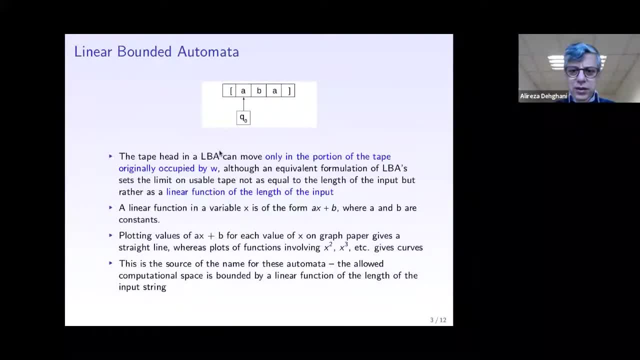 linear. I hope in the next slide it is available. but one, yeah, I'm curious to mention that. okay, so the tape head can move only in the portion of the tape originally occupied by W. W is the input string. although an equivalent formulation of LBA set limit. you sets the limit on usable tape not equal to. 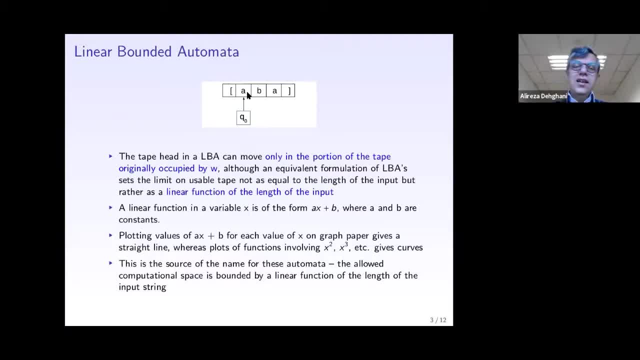 the length of input rather than a linear. so we say for the LBA, the area of the tape you can use is exactly the same size as the string, as you can see this image in this picture. okay, but that's not the case, since it is called linearly the area. 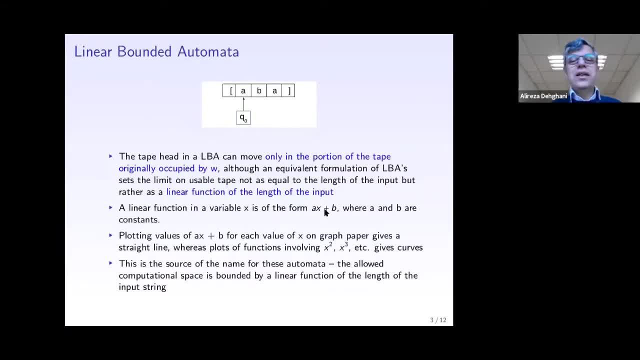 that you can talk about is linearly dependent on the length of the string. so if your string is X, the area that you can have could be A, X plus B. you remember? that's the definition of the linearity, right? so, for example, if your string is three, the length of the string is three and A is two. for example, B is one. 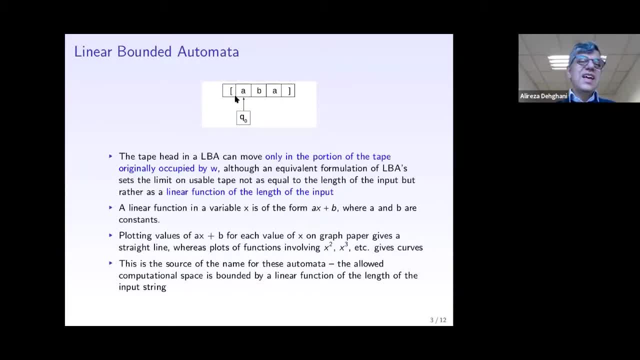 one, so it could be two times three plus one would be seven. so it is again bounded, but it is seven. it's not exactly the same fixed size as the length of the string, right, so it is allowed, then, so bounded. why? because we have end marks in here. it is bounded the area of the tail we can work on. 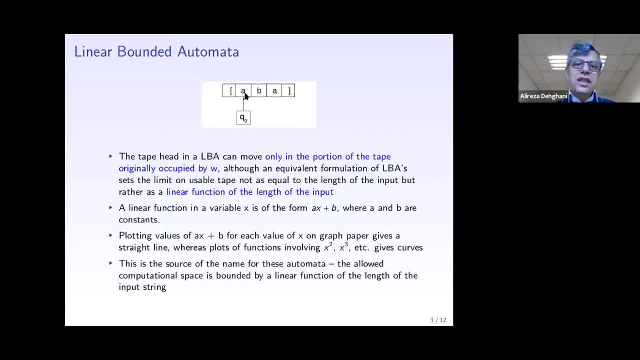 it is linear. why? because the length of the area that we can use is exactly linearly dependent on the length of the string. it tries to justify what is the difference between the linear and, you know, the other shape of functions. you know that. i don't need to go through that. this is the. 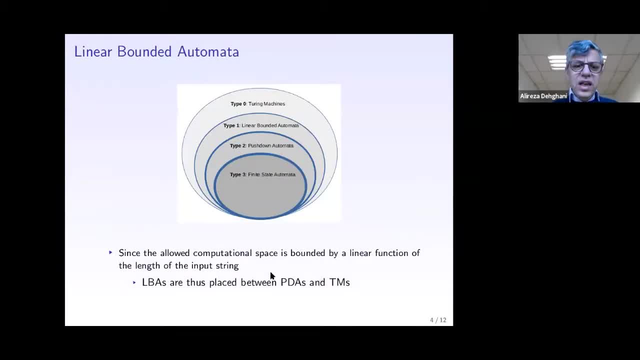 source of the name for this automator. okay, and, like i said, since it is the allowed computation, space is bounded by a linear function of the length of the input. lbs are thus placed between vd, pdas and pm turing machines. okay, so, as you can see, it is really very similar to the turing 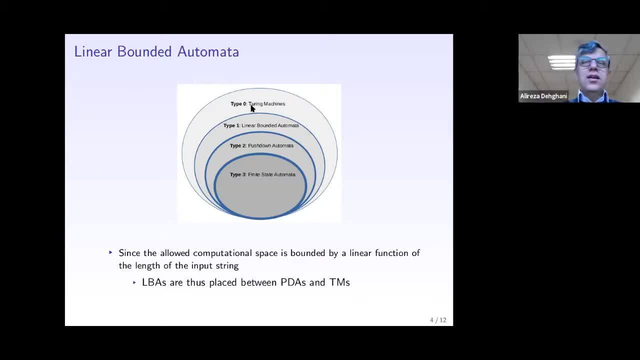 machine in the sense of it can write, it can read, it can move right length of the string. it tries to justify what is the difference between the linear and the other, left and so on, and from the other aspect it is very similar to the other machine. it has final. 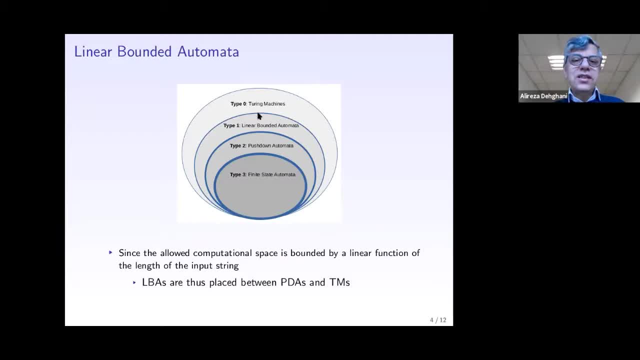 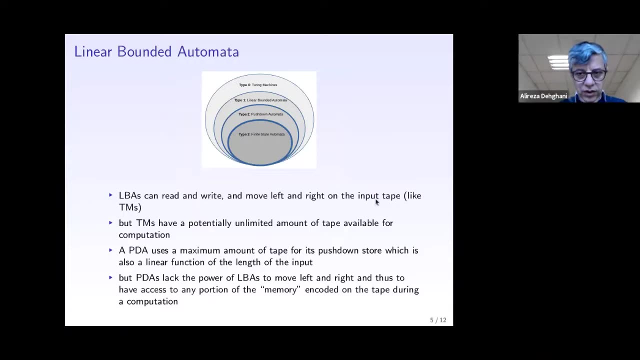 state, a finite number of state, and also it has sort of the final state, initial state, instruction, everything. so it is a machine automata that can sit between pda and turing machine. lbas can read and write and move left and right and the input state but turing machine have a potentially 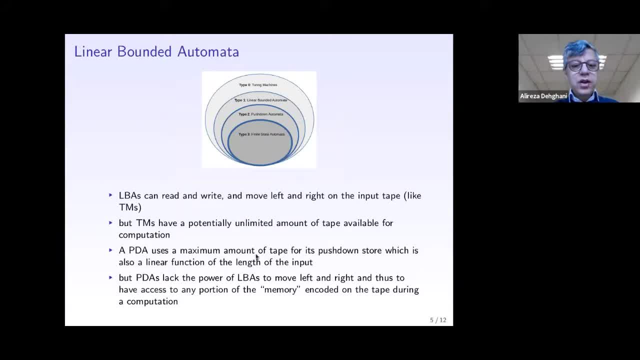 unlimited amount of tape available for computation. a pda uses a maximum amount of tape for its push and store, which is also a linear function of length of. okay, we are trying to compare them here, but pds lack the power of lbs to move left and right. 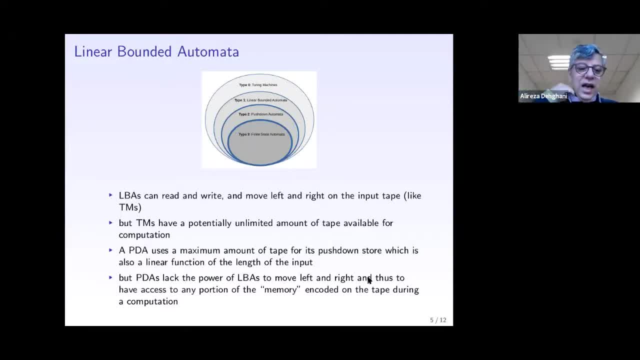 that was the difference. i may ask: what is the difference between pda and lba? one of the difference is: uh, pda cannot move left and right and also it cannot um, and thus to have access to any portion of the memory encoded to the tape during the computation. so that's the reason why. 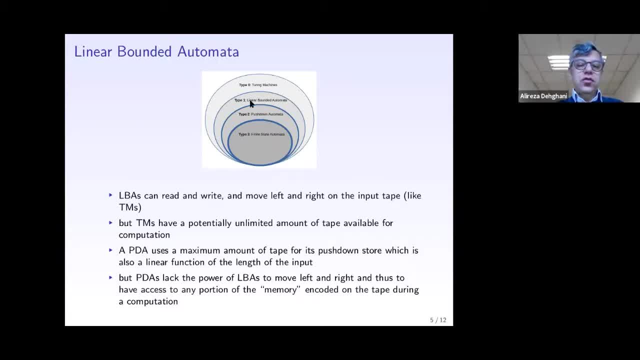 lba is stronger, more powerful machine that pushed on automate and touring is more powerful because you have the whole tape available for you to do anything you want. so you see, for some problems maybe if you want to check the things, you need to go, move to the right, move to the left, forward, backward, quite a few times to do something. 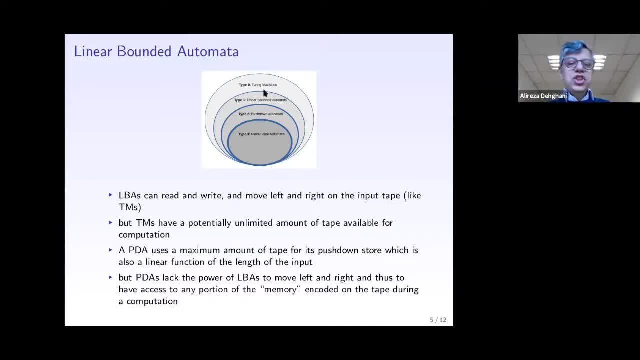 so if the language you want to work with the machine is really more complicated, touring machine will give you more capability, more flexibility, more power to do the stuff. so that's the reason why touring machine is a more powerful machine than the lba and it is more powerful than the push. 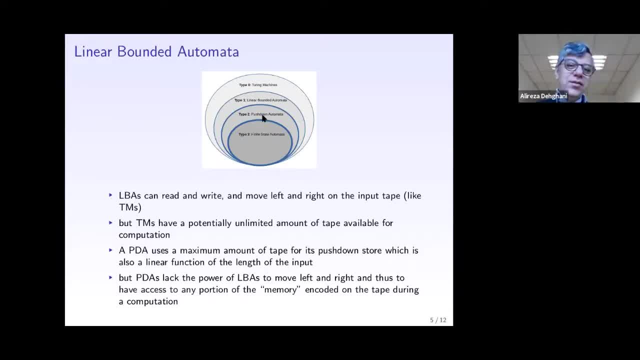 down automata. in push down automata we cannot move left but we have stack. so that's kind of facility makes the machine more powerful and in this case it is less. it has the less power among all the machines because there is no external memory. it's not possible to write. 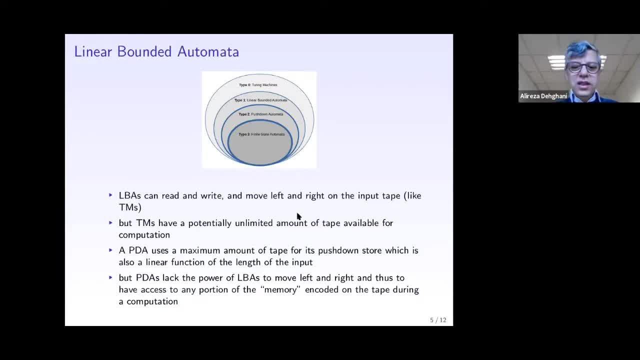 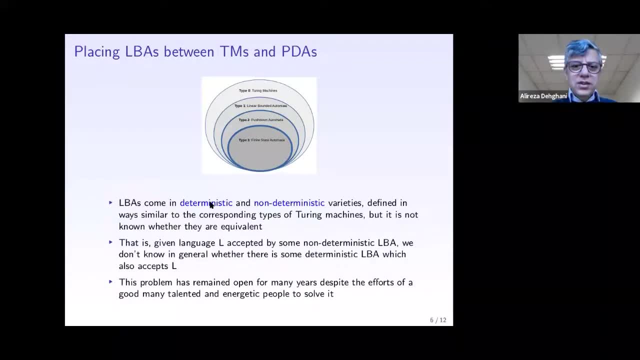 it's not possible to move left and so on. okay, the level of machine is limited, and so on. so actually we are comparing the chomsky hierarchy one more time. so lbs coming deterministic and non-deterministic variations defined in a very similar to corresponding type of machine, but it is not known. 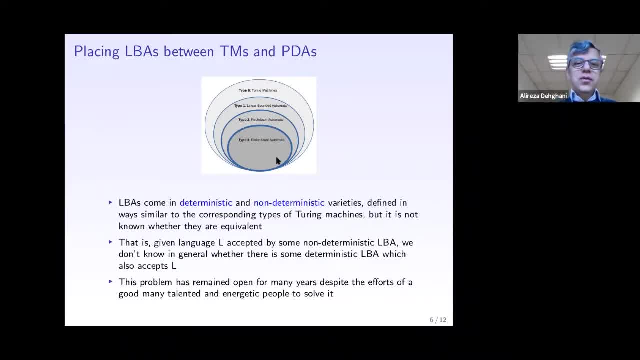 whether they are equivalent. what does it mean? it means, if you remember, for example, in finance state automata, we say: if that's a non-deterministic machine automata that does something, for that we can find a non-deterministic machine automata that does something. for that we can find a non-deterministic machine automata that does something, for that we can find a. 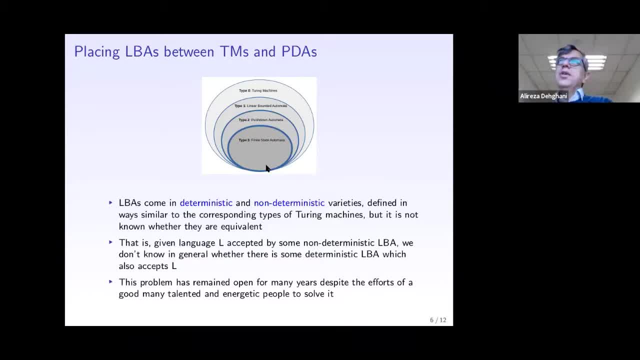 deterministic machine, or in other words for any deterministic finite state machine, at least we can find at least one non-deterministic one which are equal both of them. but that's not the case for lba. that means that is given language l accepted by some non-deterministic lba. 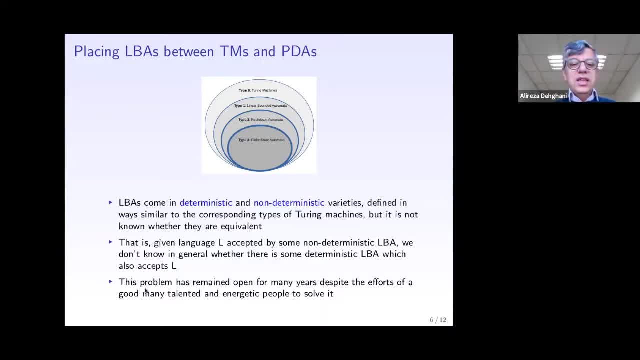 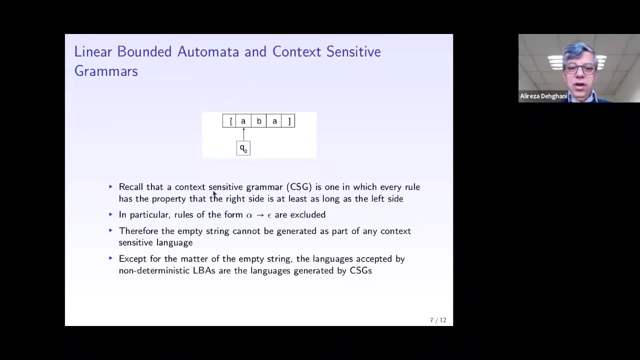 we don't know in general whether there is some deterministic lba which also accept them. okay, so this problem has remained open for many years, despite the effort for a good many talented and energetic people to solve it. and recall that the context sense is sensitive grammar. you remember, for each specific automata we had three different parts. we had the automata, we 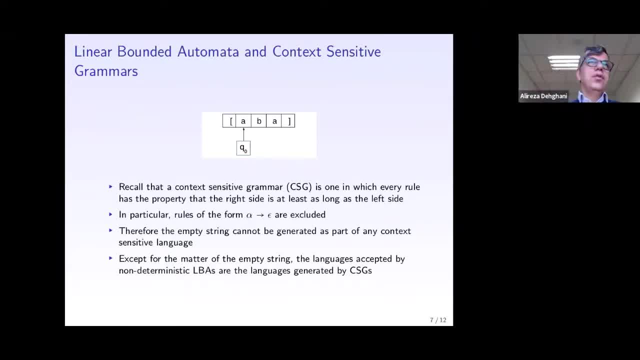 had the grammar, we had the language. okay, for example, for finite state automata, we had the regular language and regular grammar. okay, for the pushdown automata, we had something similar for the lba. we have the same, so it is lba. we have the same, so it is context, context. 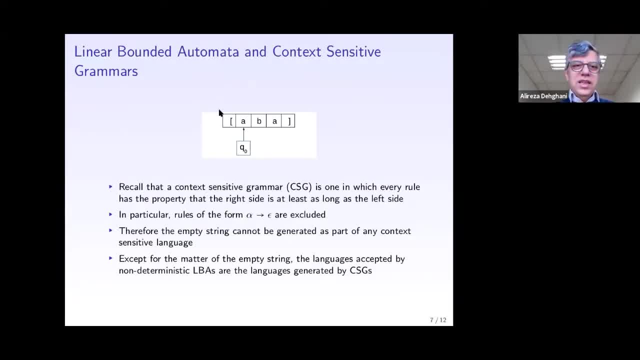 context. sensitive grammar is the grammar related corresponding to linear bounded automata is one in which every rule has the property that the right side is at least as long as the left. so you remember, in week number two, if i'm right, i think so, yes, i think yes. so at that time, if you, 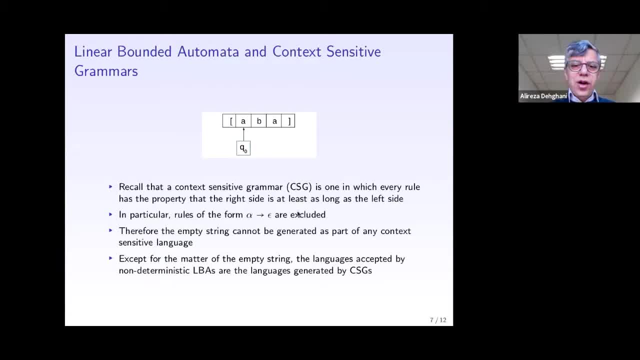 remember we try to define different types of the grammars at that time. for the context sensitive grammars we say the right hand side should be the context sensitive grammar and the right hand side shouldn't be the length of the right hand side in any instruction shouldn't be smaller than the. 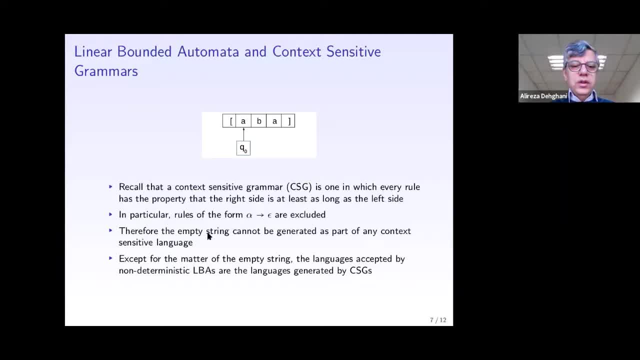 left hand side in particular. so let me see the word in here, so it's not sharing cable. then, in particular, rules of the form alpha to empty or epsilon are excluded, so it is kind of shrinkable. you are getting one string or something in the left hand side and you're delivering nothing. so 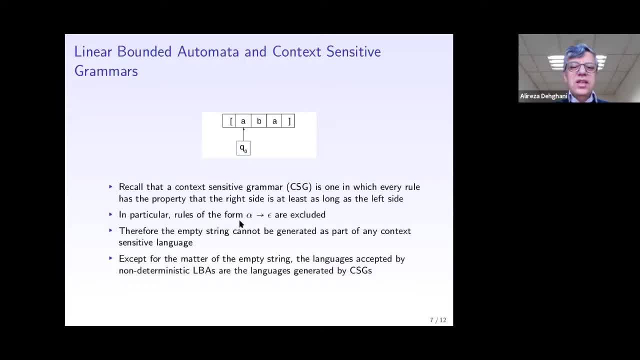 that means you are trying to shrink the uh, the input in the machine, so it's not included in context sensitive grammar and therefore the empty string cannot be generated as a part of any context sensitive languages, except the matter of the empty string, the languages. so while we are talking about dandy, so like i said, 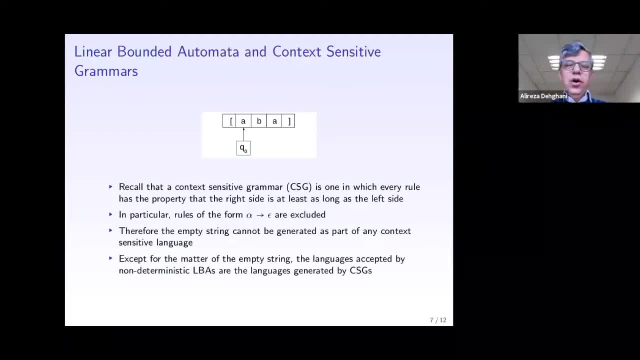 for any. you know we have three different pieces, three different parts: the automata, grammar and language. right, and i said we can make a correspondence between all of them in each level of the chance. how do you think you should address that to the context? sensitive grammar. well, if you can't address that in this worst case scenario, you have to talk about it and 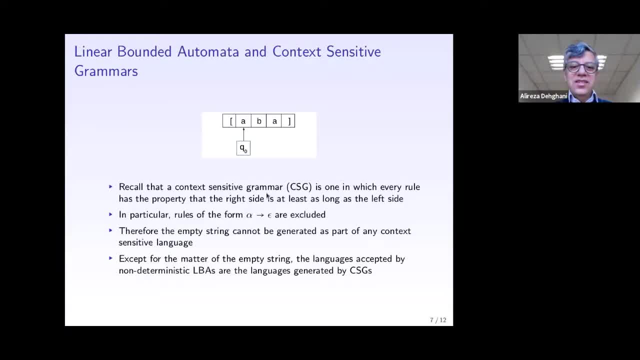 you need to make a conversation with the context sensitive grammar. so if the context sensitive grammar is not available, then the context sensitive grammar has to be separate from the context sensitive grammar, right, and you know, it's also possible if the context sensitive grammar is non-existent. hmm, i feel like our language is not available yet. yeah, yeah, yeah. 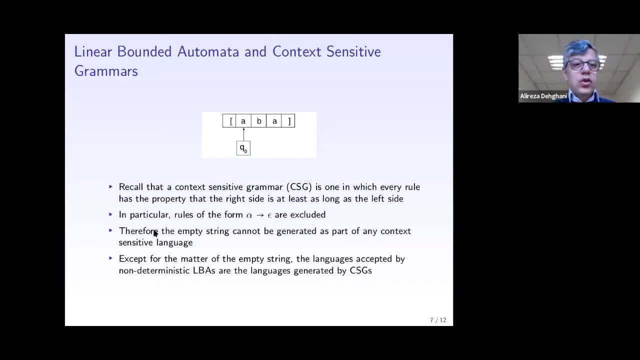 while the linear bounded automator can do that. so if you want to make a correspondence between them, then, except for the matter of the empty string, the language accepted by non-deterministic lvas are the language generated by csg. so it is possible. it could be a good case to ask. 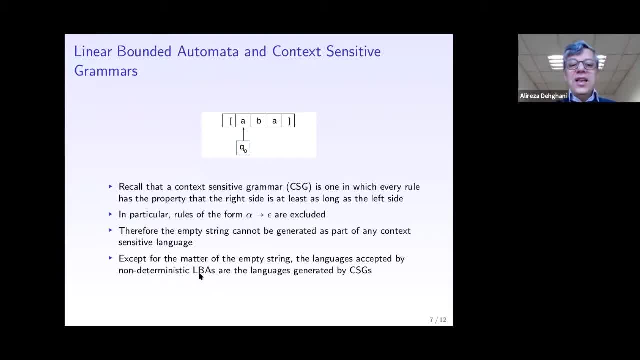 a question for in the final exam. so in lva and lva could be corresponding to cgs. if we exclude the matter of generating the empty again. let's read it again. except for the matter of empty string, the language accepted by non-deterministic lvas are the languages generated by csgs. given a csg, 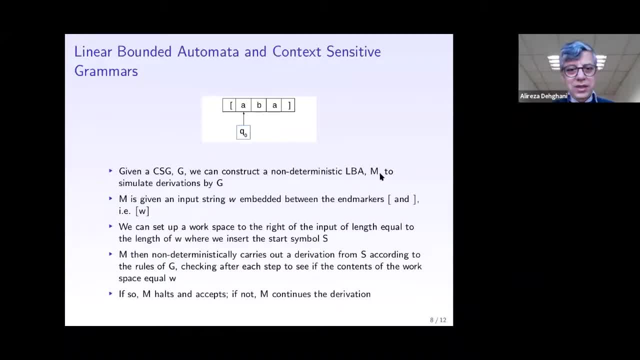 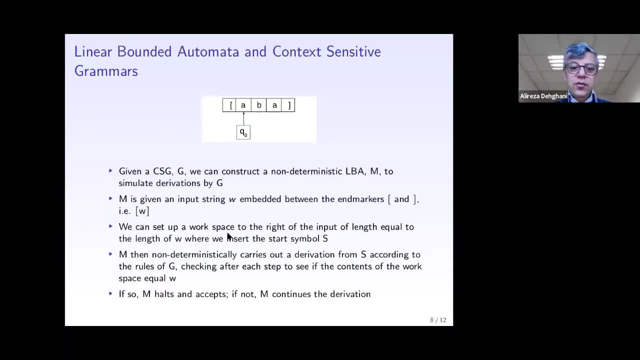 marks something like that. we can set up a worker space to the right of the input of the length equal to the length of the w, where w insert the start symbol m, then the non-deterministic carries out the derivation from s according to the rules of g, checking after each step to see if the contents. 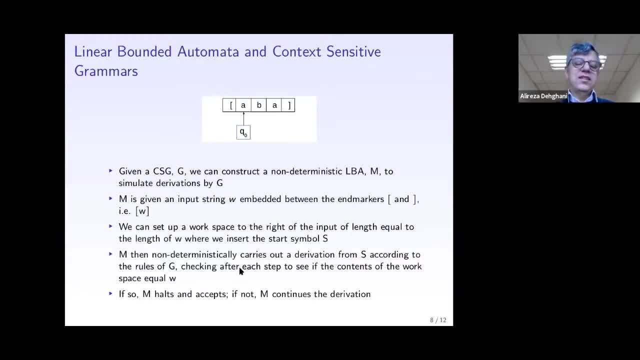 of the work is basically called w. if so, m halts and except it tries to show you how a linear bounded automator can accept or reject the machine. it's very similar to turing machines, right? you start from a starting symbol in here and then you walk through that and then 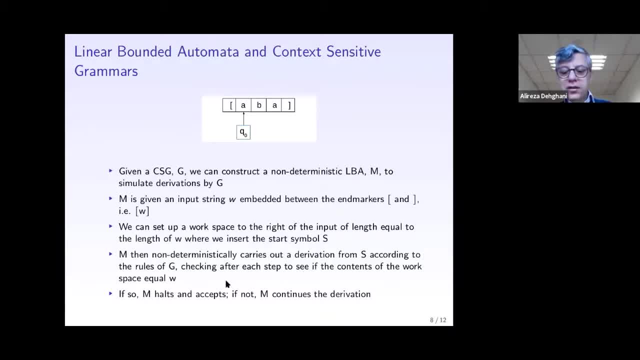 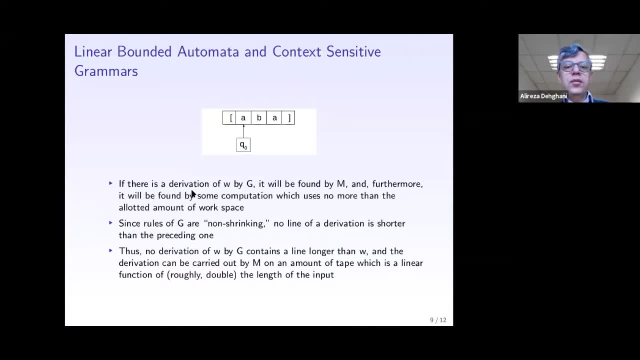 at the, at some situation, you halt somewhere and then you accept the string. if there is derivation of w by g, it will be defined by m and furthermore, it will be defined by some computation which uses no more than the allowed amount of the word space. since rules of g are non-shrinking, no line of 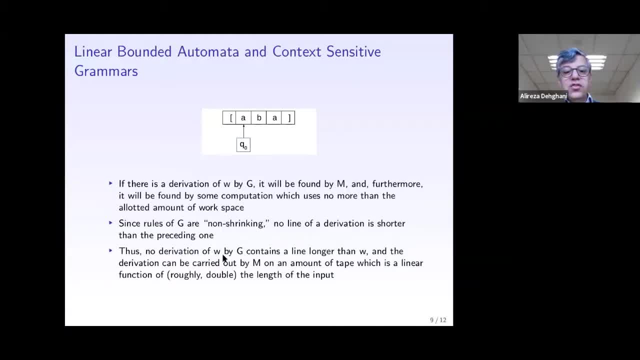 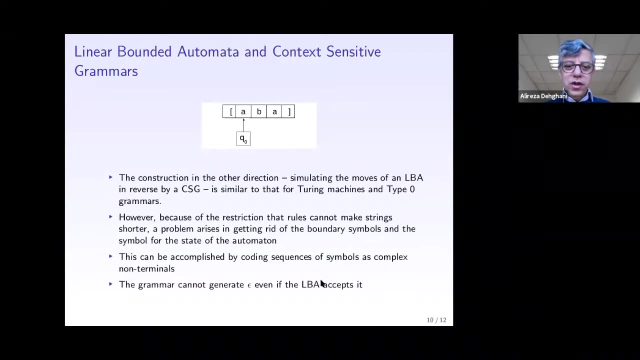 derivation is shorter than the preceding one. thus, no derivation of w by g contains a line longer than w and the derivation can be carried out by m on an amount of tape, which is a linear function: the length of the input right in terms of time, complexity, the 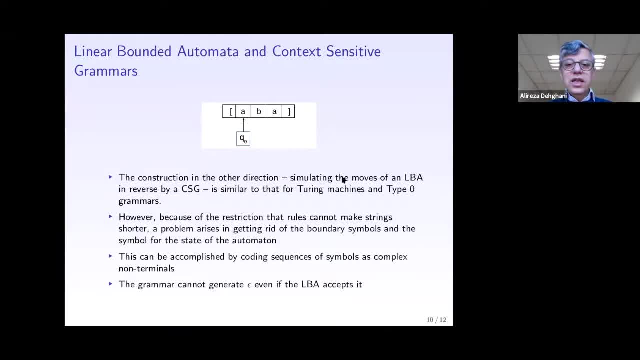 construction in the other direction. simulating the moves of an lva in reverse by cj is similar to that for turing machine and type 0. however, because of the restriction that rules cannot make a string shorter, a problem arises: getting rid of the boundary symbols and the symbols for the state of automation. this can be accomplished. 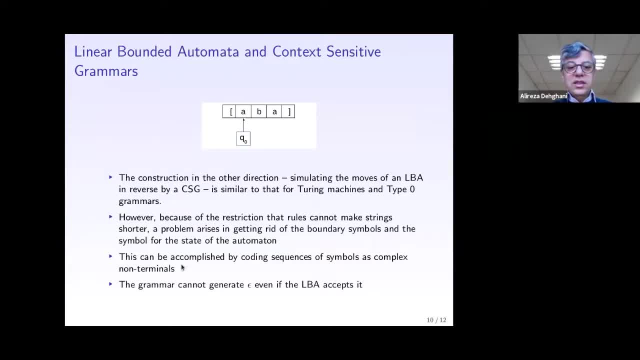 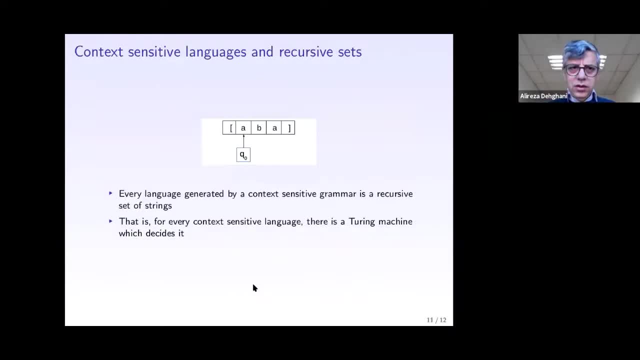 by coding sequence of symbol as complex non-terminals, the grammar cannot generate it. that's the whole thing, actually, i discussed what i read through the whole thing. context sensitive recursive sets. every language is generated by context. sensitive grammar is a recursive set of strings. that is for every context, cs, context sensitive languages- there is a turing machine. why? because context. 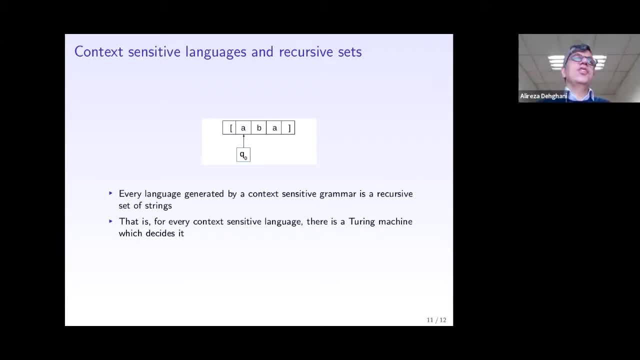 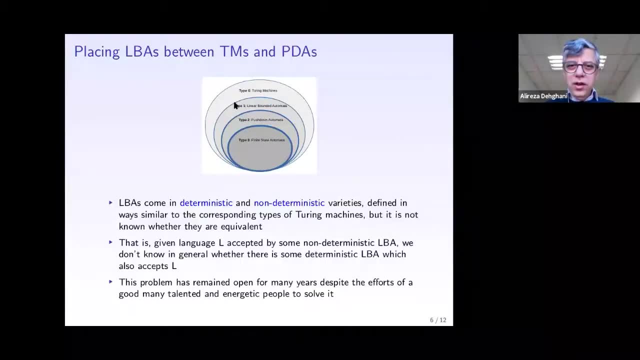 sensitive languages and grammars are a subset of the turing machine. in the hierarchy back in here see this: linear bounded automata are a subset of turing machine. linear bounded automata can be corresponded, can be related to the context: sensitive languages and grammar. that means every. 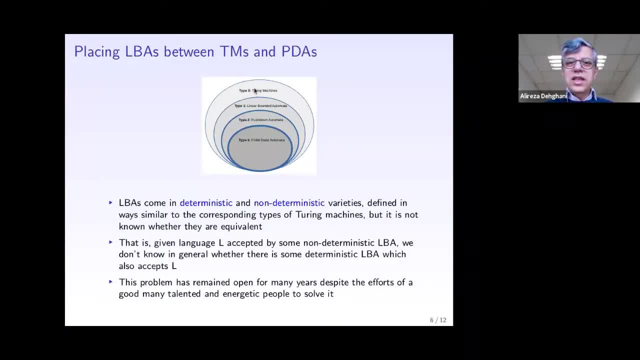 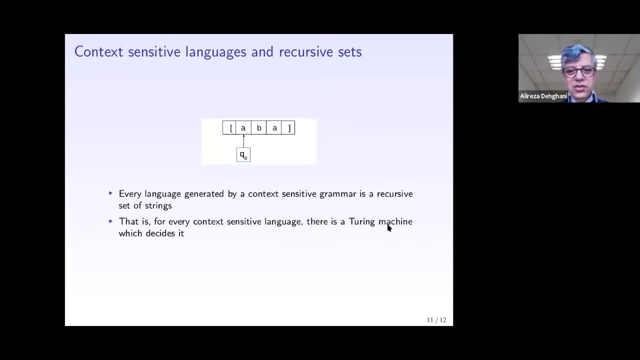 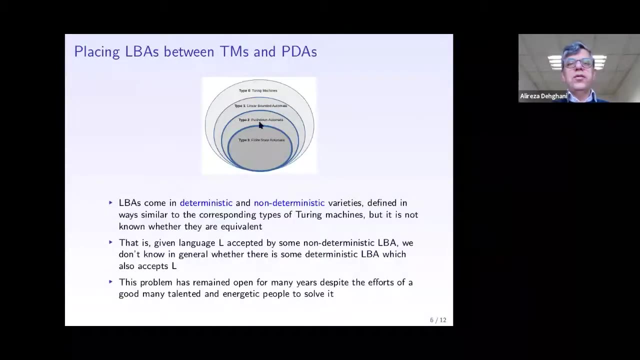 context sensitive languages and grammars can be related somehow to the turing machine because that's a subset of that. okay, for every context sensitive languages there is a turing machine which decided it is possible because that's a subset. you know the meaning, the definition of being a subset. 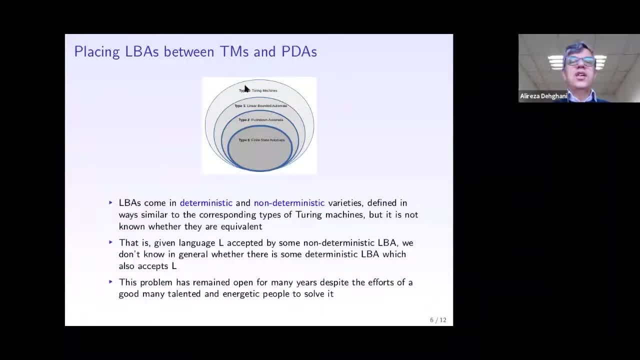 if this guy is subset of this guy then probably using a machine from this category we can deal with some languages inside this part. but the other way around is not correct. i mean we cannot find the, we cannot find the machine in this category that can work on the languages and string inside. 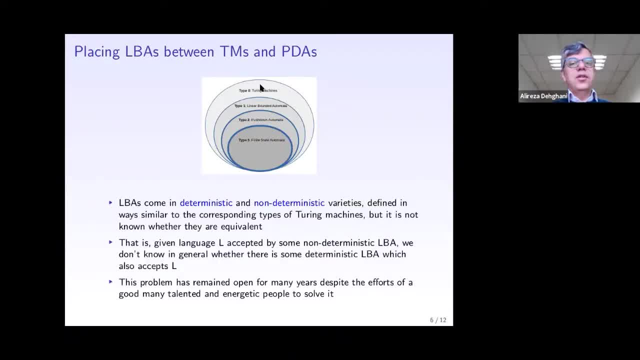 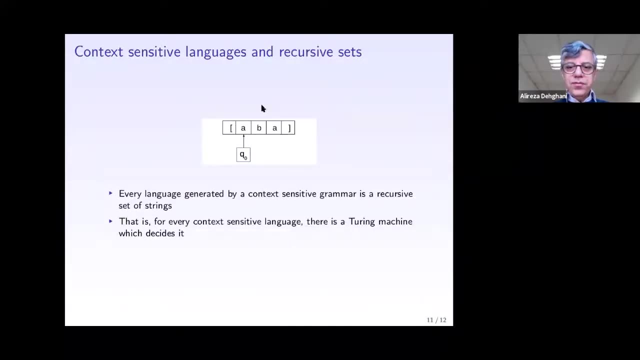 this category. so since linear bounded automata is a subset of turing machine, in other words, since context sensitive grammar is a subset of this grammar enumerated languages- so that means we can have a turing machine that decides any context sensitive languages and that's the whole correspondence. again, i think that's the main point, that we do deal with the altex. 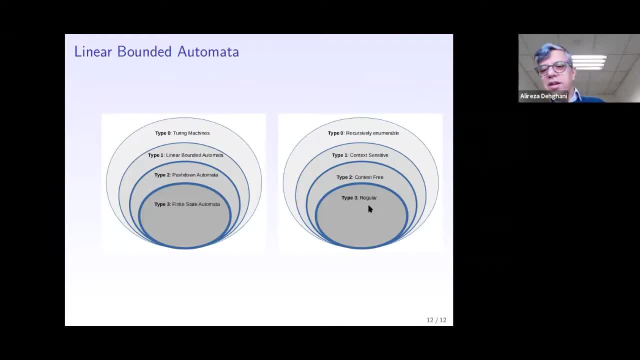 as unclear方 of is a这个 yi 一般して infinite state automata, regular languages. what relates these two things together? the grammar, regular grammar, we have the context-free languages, we have the pushdown automata and the context-free grammar. correspond these two, these guys together: linear bounded automata and context sensitive? 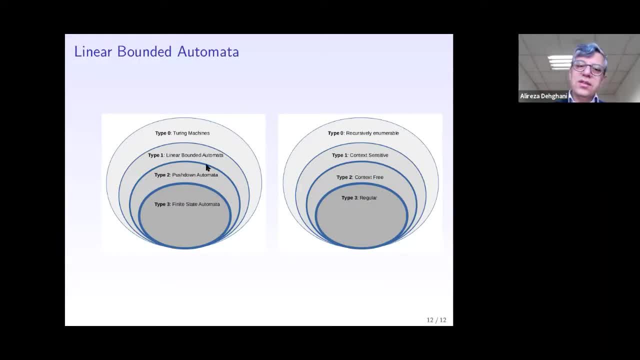 languages. again, the context sensitive grammar relates and corresponding them together and recursively in your label languages using the corresponding grammar is connected to turing machine. that was the whole hierarchy of definition.